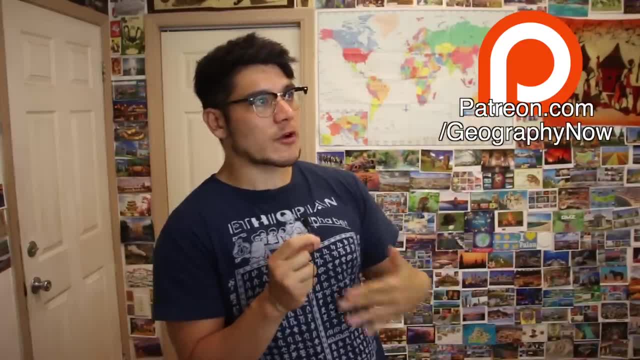 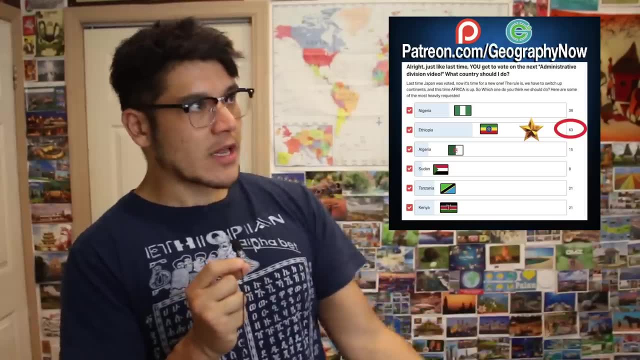 So, as you know, people on patreon get to vote for the next filler week for administrative division videos, and the rule is we have To switch up the continents. this time It's back to Africa. I asked you guys to vote from some of the top selections and you guys voted for. 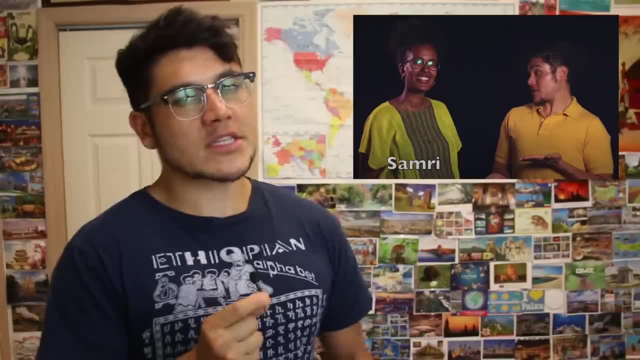 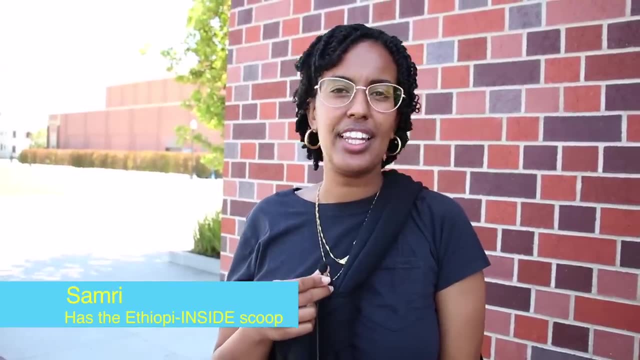 Ethiopia. remember, the Ethiopia episode is really great. I really wanted Samri to be in this video but she couldn't make it. but she sent you guys a little message. Hi everyone, Thank you so much for voting for Ethiopia this week. Sorry that I can't be with you in this video. 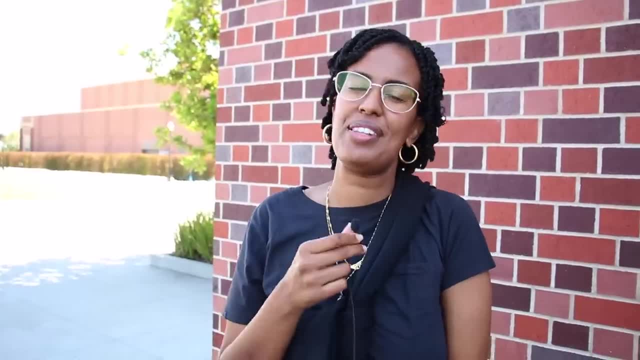 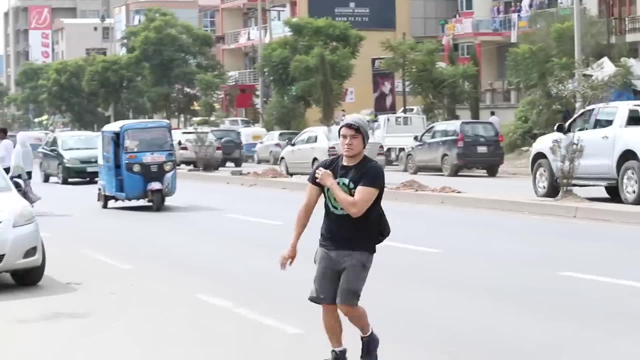 But I hope that you get a lot of information and learn a little bit more about this amazing country. Thank you. Thank you, Samri. Now. I had the very fortunate experience to actually go to Ethiopia last year with Caleb. We had a layover in Addis Ababa. I met up with Abdul, one of our subscribers- really awesome guy. 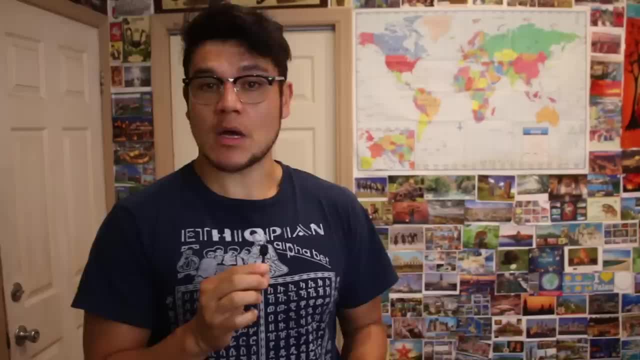 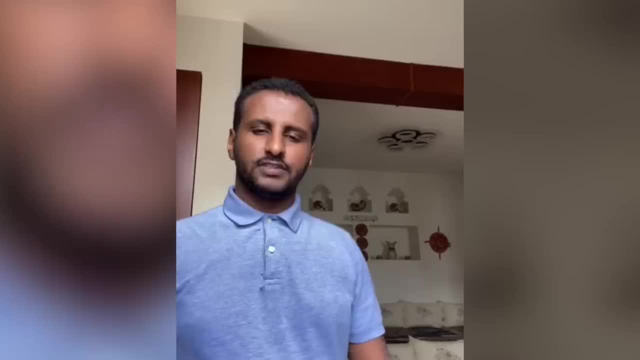 I actually reached out to Abdul to see if he'd like to be in this video. He said yes. Abdul, say hi. Hello, this is Abdulahi from Ethiopia, land of origins. I met Caleb and Paul last year While they were visiting Ethiopia. thanks, Abdul. for those who don't know, Ethiopia kind of has like a very reputable position in the African continent. 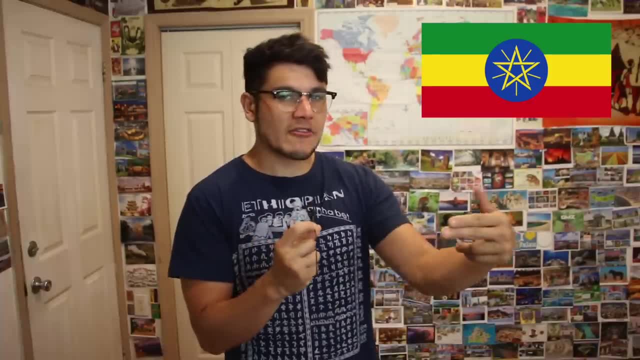 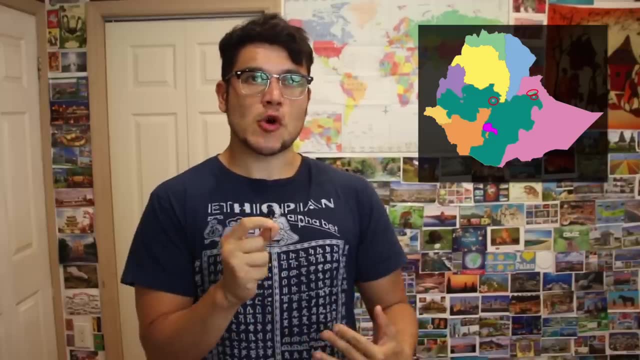 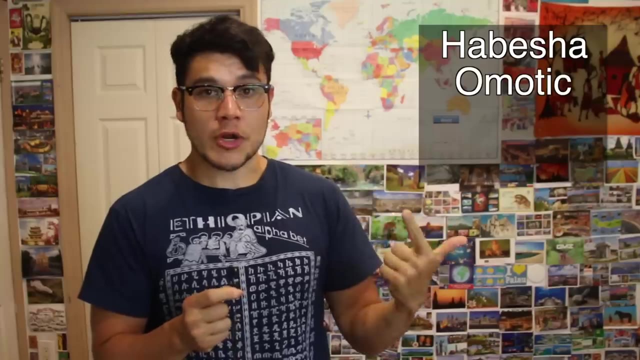 It was never fully colonized like the Italians took a stab at it for like five years, But it didn't really work out. fascinating place, both in the city and the countryside, and what's even more interesting is that each region of Ethiopia has such a Fascinating story. in contrast with people, groups and languages, have four main ethnic families: the Habesha, Omotic. 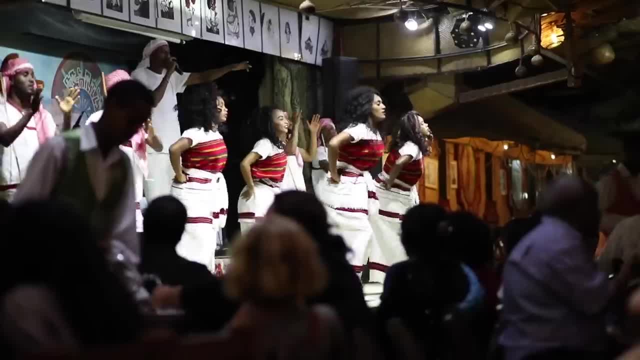 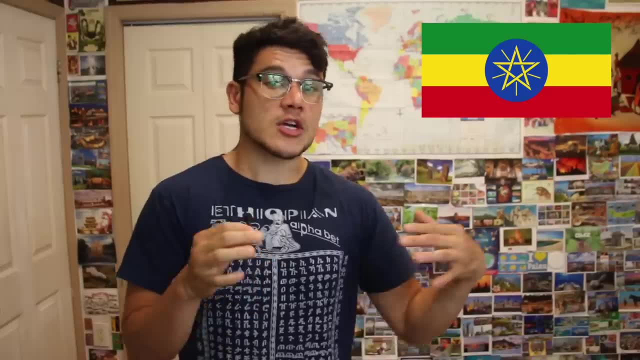 Nylotic and Cushitic. you can travel less than 20 miles and find a completely different people group with a different Writing system and language and cultural tradition than the one that you just passed through. It's amazing how the country holds itself together today. There are ten regions, or Kili, keep in mind. actually, in June of 2020, 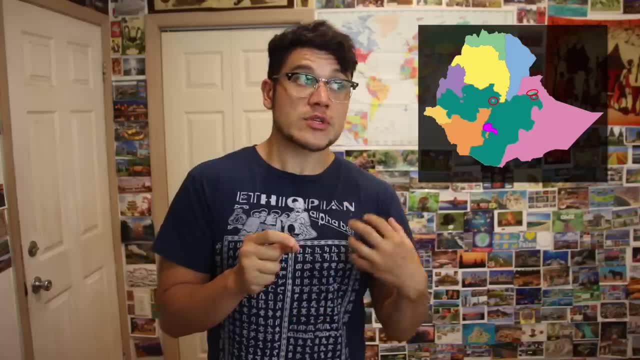 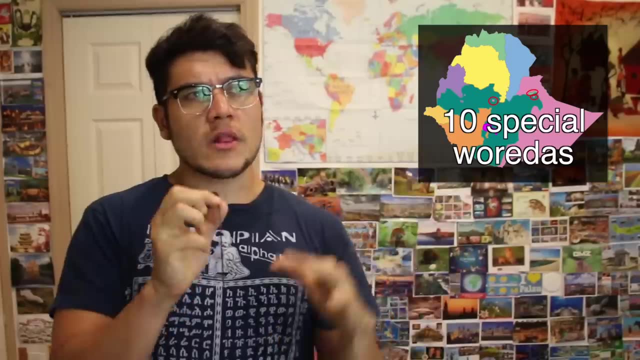 The Siddhama zone actually got upgraded into a region, making it the newest region, and in addition They have two charter cities which act like regions, and on top of that you have ten special warredas, Which are like districts within the regions, that have their own autonomy and don't act the same as the regions. It's confusing. 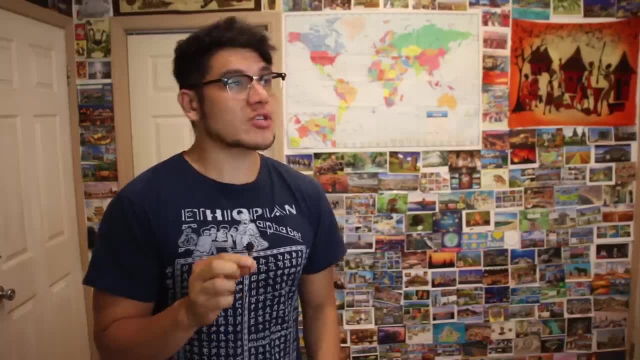 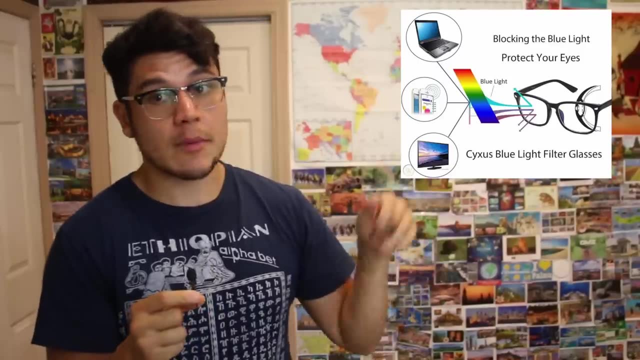 Here's a list of all ten of them. We don't have time to get into it. All right, And before we jump into it, just want to mention that this episode is brought to you by Syksis glasses, the blue light blocking glasses. if you're like me and you spend a lot of time on the computer or laptop. 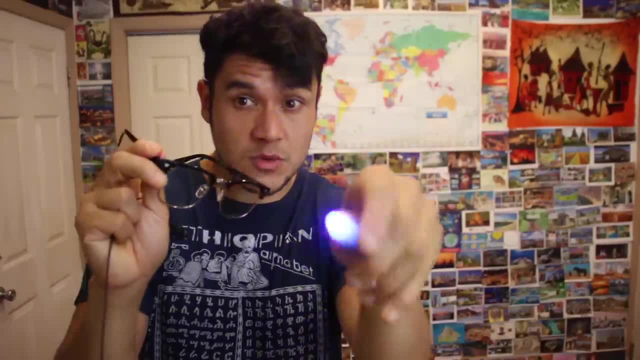 Sometimes you get a little bit of eye strain. Syksis hooks you up. each pair of glasses even comes with this blue Right light ray that you can test on the glasses. really cool stuff. And even if you don't even care about that stuff, the glasses look cool too. 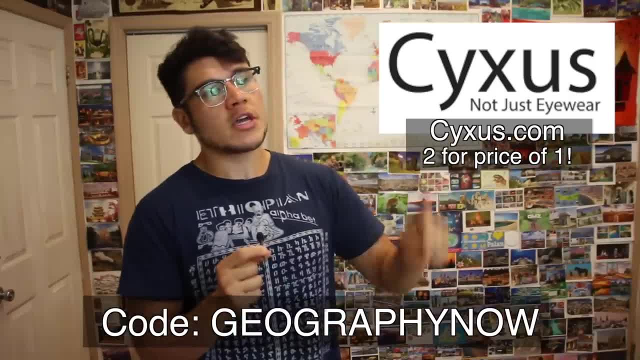 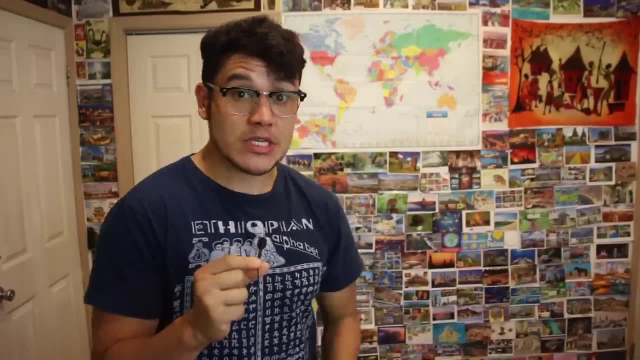 Anyway, and right now, if you go to Syksiscom, you can get two for the price of one if you use the code Geography. now, Syksis, you guys rock. Thank you so much for sponsoring this video. All right, and let's jump in. now to the regions and charter cities go. 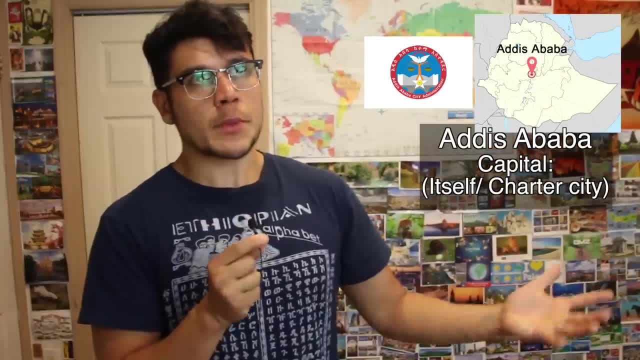 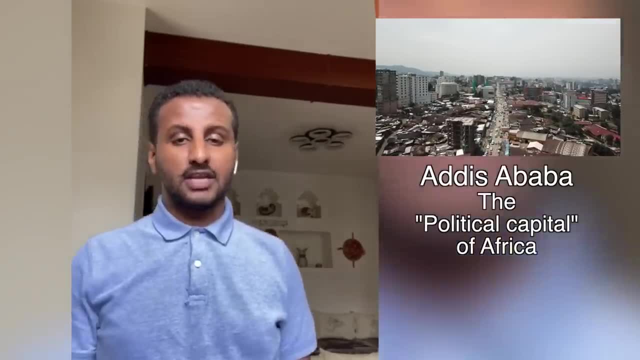 the first one, Addis Ababa, the national capital of Ethiopia, Abdul, take it away, I decide, was definitely unique city is often referred to as a political capital of Africa for its historic and diplomatic significance. I mean the UN Economic Commission for Africa and the African Union headquarters are located here. 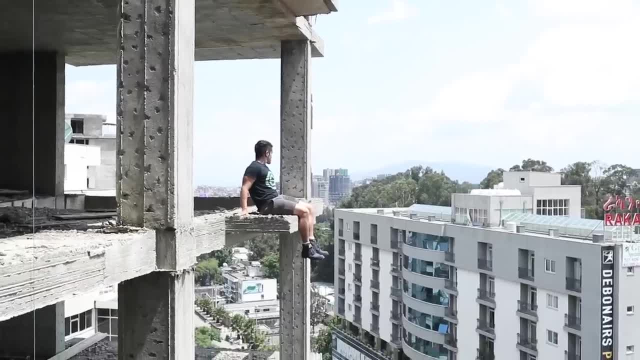 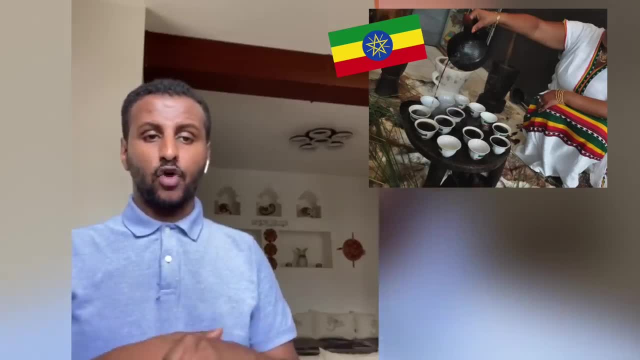 This is a very fast-growing city, with skyscrapers popping up everywhere, And it's a bustling city, with random horses in the street as well as coffee stores everywhere. Remember, coffee did originally Come from Ethiopia and in 2015 we built our first life real system and overall. 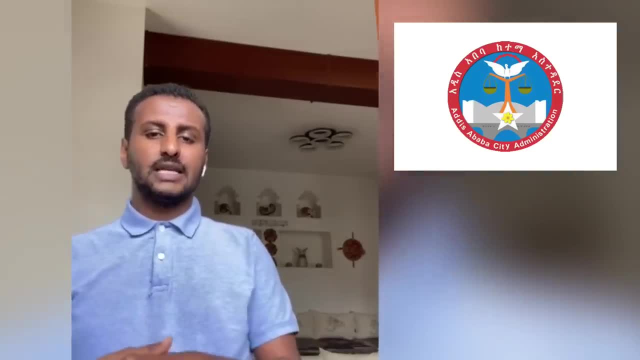 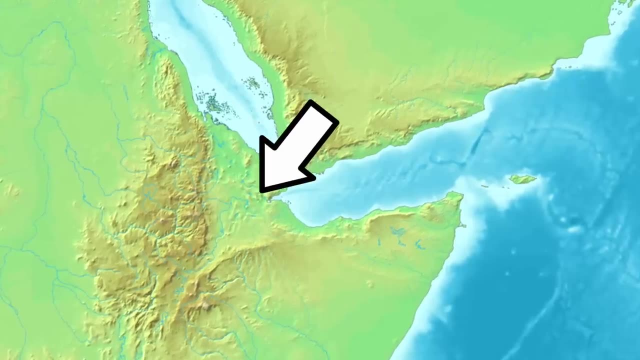 I saw this, The gateway and hub to Ethiopia, both domestically and internationally, afar capital, Samara. Okay, So, basically, if you look at Africa from space, you'll notice that there's like a deep triangle shaped valley that juts into the East horn Side of Africa. Well, that area is known as the afar triangle. 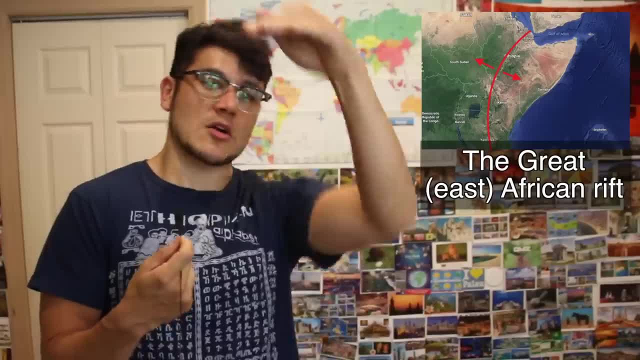 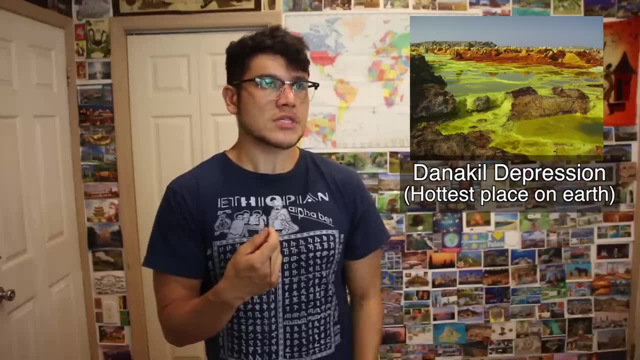 It is basically the beginning of the great African rift that cuts all the way through the eastern part of Africa. It's a volcanic area with lots of geothermal activity. It's hot, It's dry. It even has the hottest place on earth: lots of really cool looking salt flats and 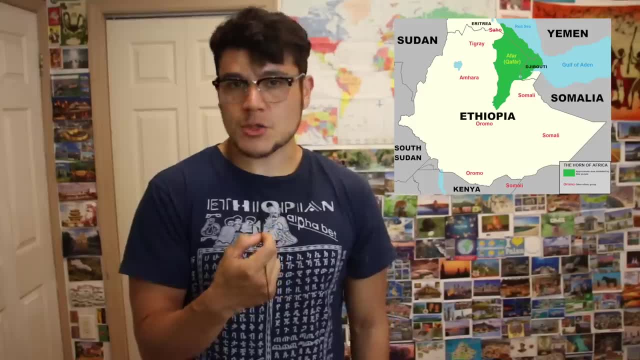 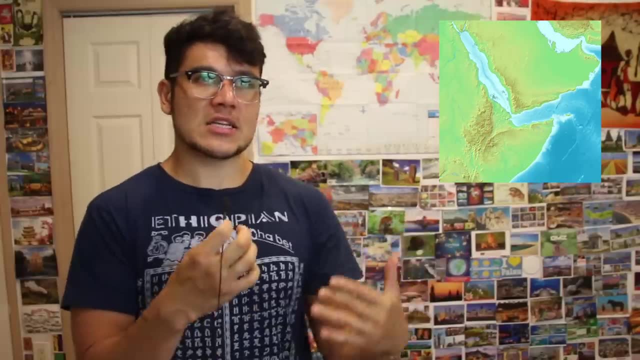 It is primarily inhabited by the afar people. whompst can also be found in Eritrea and Djibouti. the afar people are a Kushitic group related to the Somalis and historically there are kind of like the gatekeepers between the Red Sea and the Gulf of Aden. 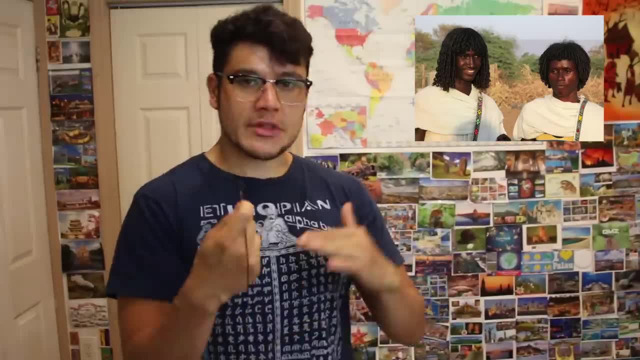 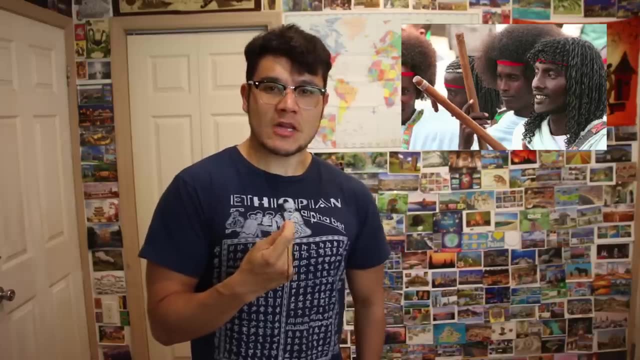 They are predominantly Muslim. They're divided into clans and traditionally They were livestock herders. Often You can see men with the curved Gelee knife. Yeah, long story short, They're kind of like the volcanic livestock people. Am-Hara, capital Bahirdar, This is a heavily influential region. 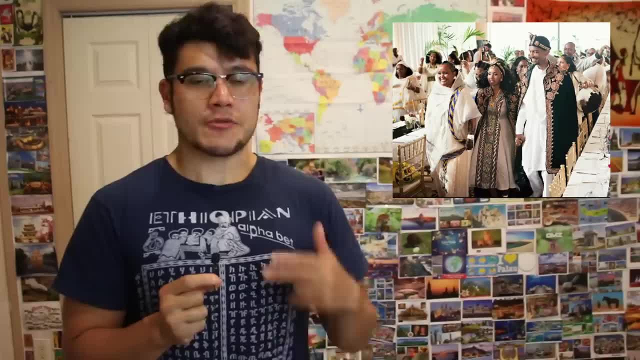 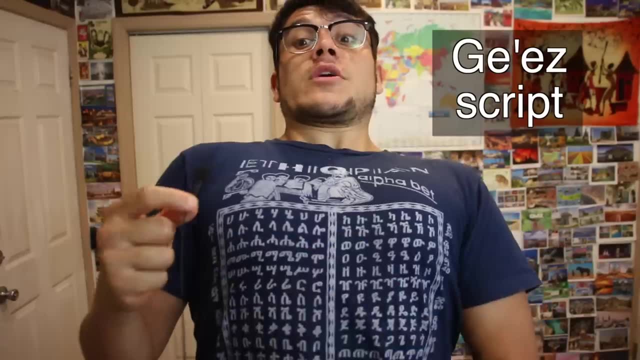 It is the second most populous region in the region, with about 20 million people and predominantly inhabited by the Amhara people. at about 90%, They speak Amhara, which is the official working language of Ethiopia. This right here on my shirt is the Amharic script. 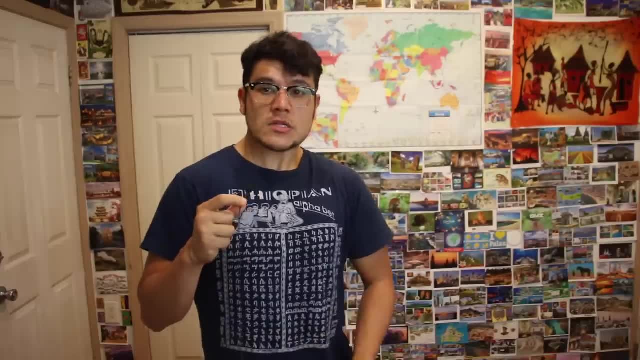 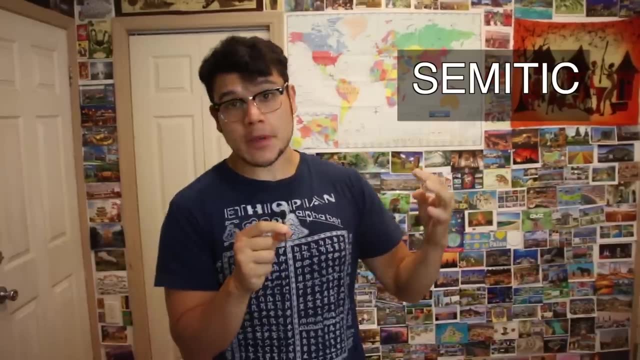 It's actually a syllabary, or abugida, of about 300 characters and it is one of the only few indigenous African writing systems And it is a Semitic language, so it is related to Hebrew and Arabic. And the interesting thing about the Amhara, along with their cousins, like the Tigre and Tigrinya people, 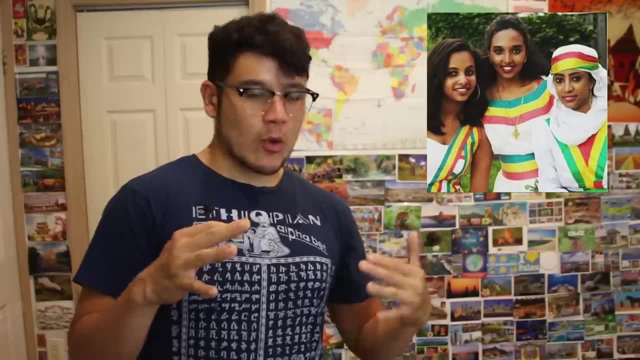 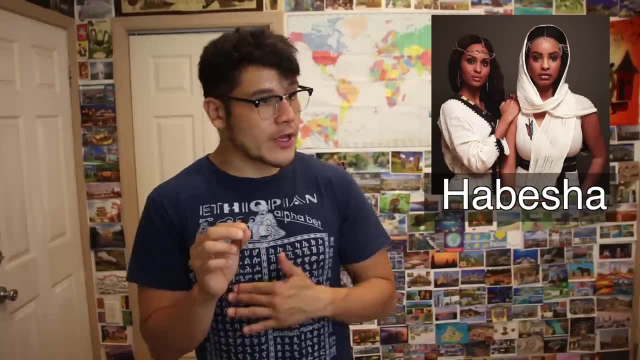 have a unique ethnic background, because they are basically what you get when you mix in Semitic peoples with black Africans and then you get a whole new people group called the Habesha. Habeshas are widely known throughout the entire African continent and they have their distinct Habesha look. 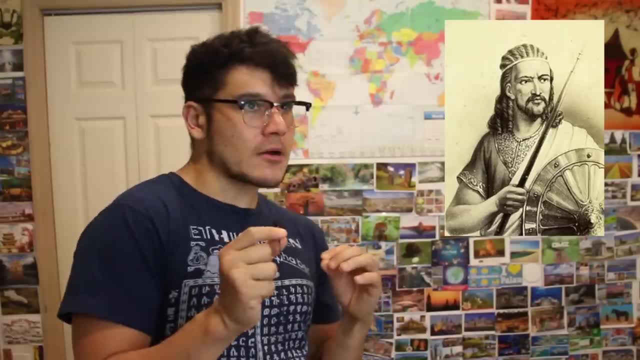 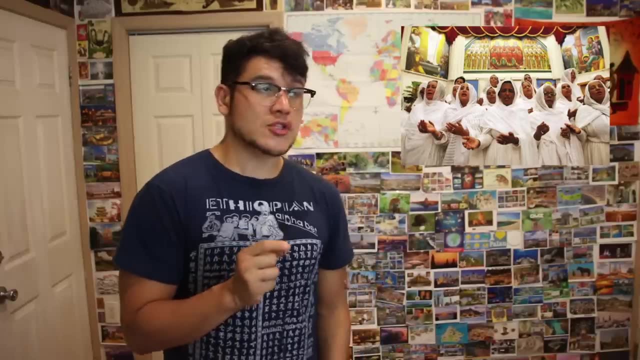 The Habesha have a long history that dates back to the kingdoms and empires from millennia ago. Their royal family claims to be descended from King Solomon in the Bible. Culturally, the Ethiopian Orthodox Church plays a huge role in Amharic households. 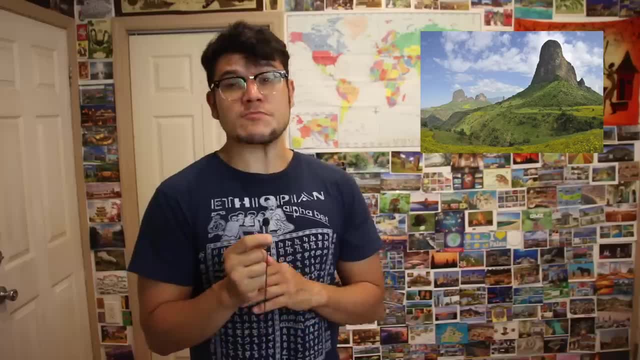 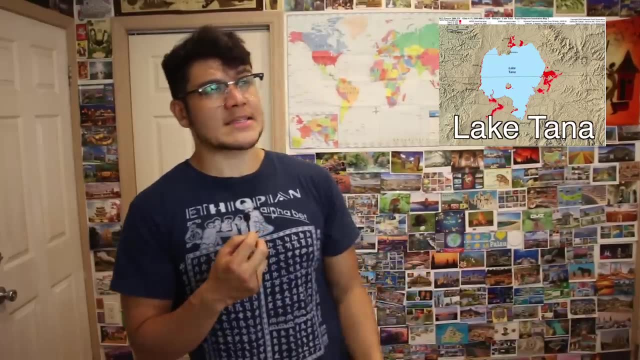 In fact, Christian faith in Ethiopia actually predates Europe. They have some of the most picturesque landscapes here: The Simeon Mountains. they have the tallest mountain in Ethiopia. They have the largest lake in Ethiopia, Lake Tana. So yeah, Semitic-based Habesha Orthodox empire culture. that's Amhara. 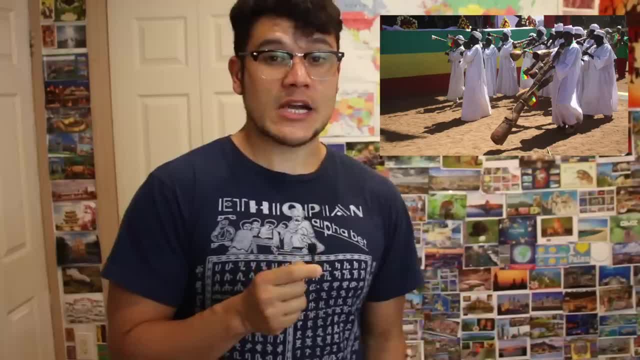 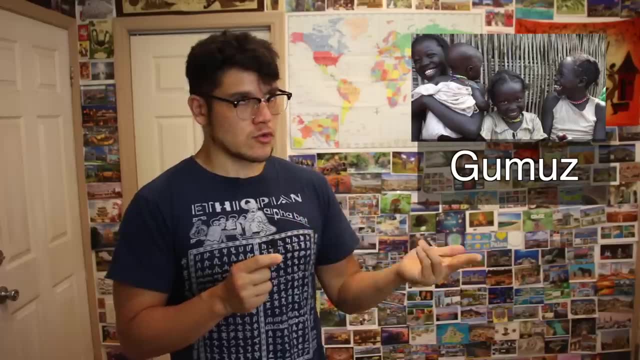 Beni Shangul, Gamuz probably butchered that Capital, Assosa named after the two people groups that live here, even though collectively they only make up about a third of the population: The Berta or Beni Shangul and the Gamuz. Both are Nilo-Saharan people groups. Basically, these people have ties to the historical civilizations along the South Nile, hence Nilo or Nilotic. It dates all the way back to ancient Nubia, which had ties to ancient Egypt As an outlier area. they've kind of struggled a little bit more with infrastructure development. 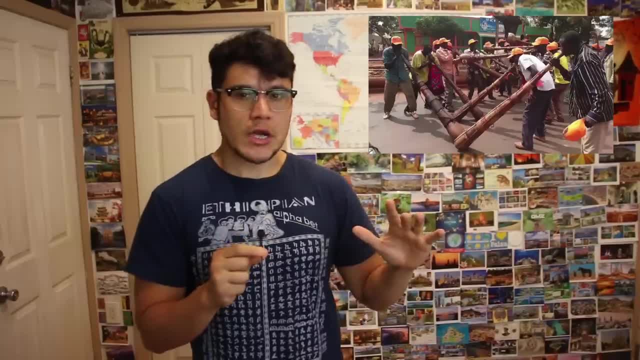 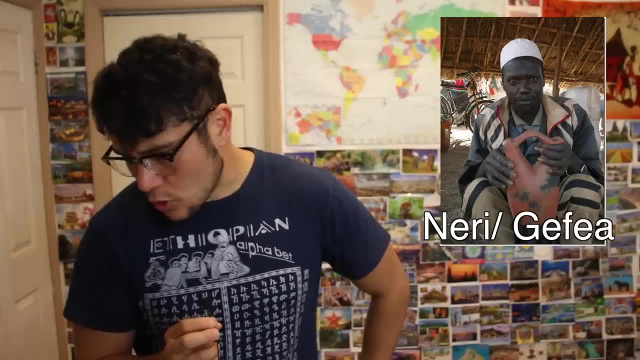 Due to the proximity with Sudan, Arabic is more commonly spoken here and Islam is the predominant religion. However, it is often synchronized with traditional customs- Let's see what I have here, Like the Neri or Gefea, which are kind of like shaman, in charge of healing rituals or spiritual issues. 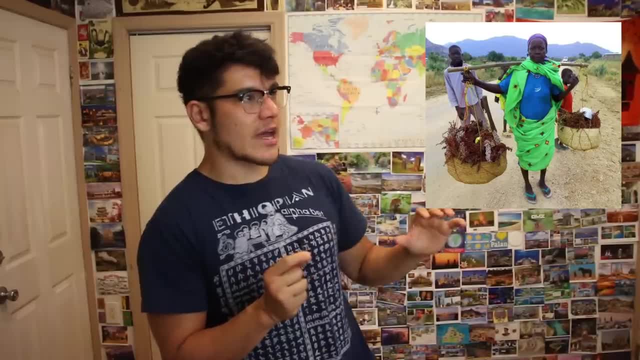 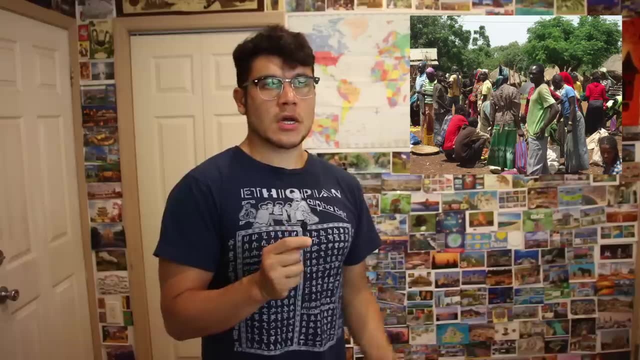 And as for the Gamuz people, they are heavy sorghum cultivators and occasional hunters. They used to be known for doing ritual scarification, but that tradition kind of died out in the past few decades. Uh yeah, rural outskirt, sometimes Arabic-speaking farmer people. 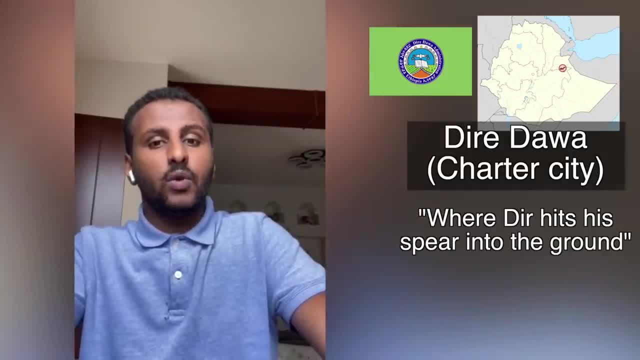 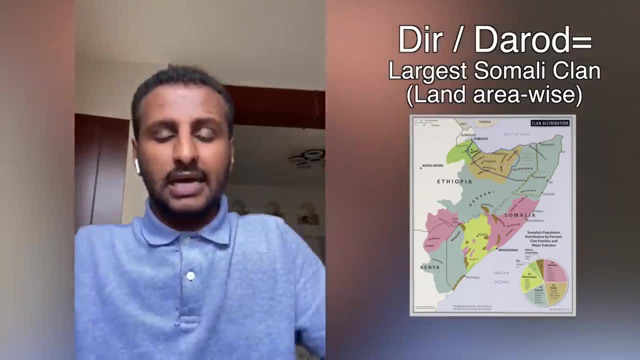 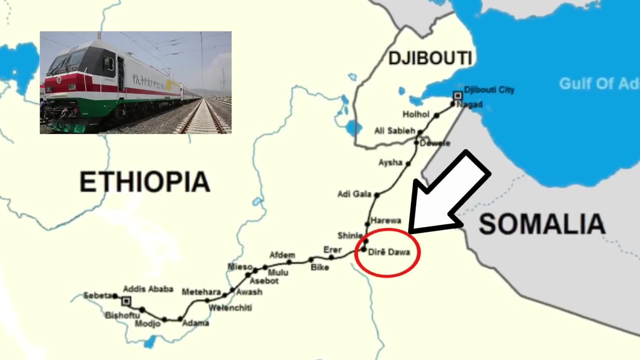 And now Abdul Dredor, the second largest city, meaning where deer hits the spear into the ground. Deer refers to the largest, most prominent Somali clan, even though Somalis are only the second highest ethnic group. The city was actually kind of constructed solely for the purpose of extending the Djibouti-Addisaba railway line. 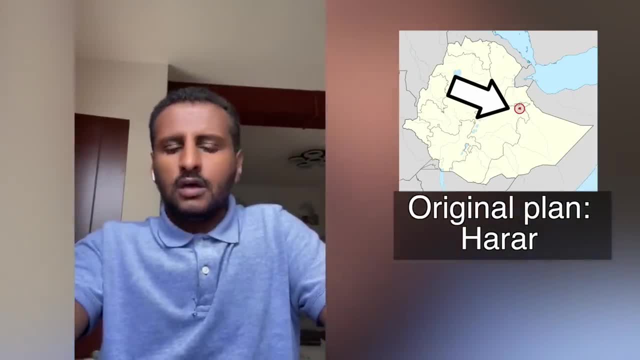 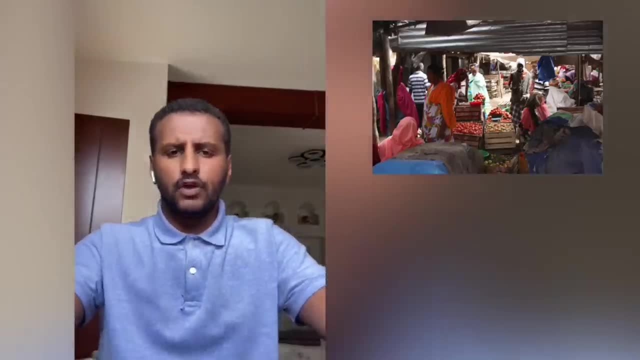 originally it was supposed to go through Hadar, but Hadar was too difficult to access in the mountains, so Dredor was created as a new level. Ethiopians from many ethnic groups flocked from all over the country and it became its own thing. 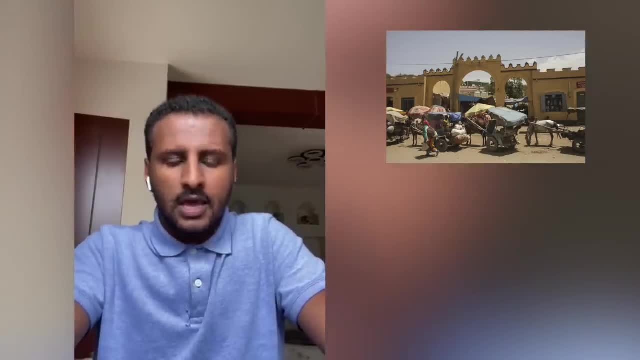 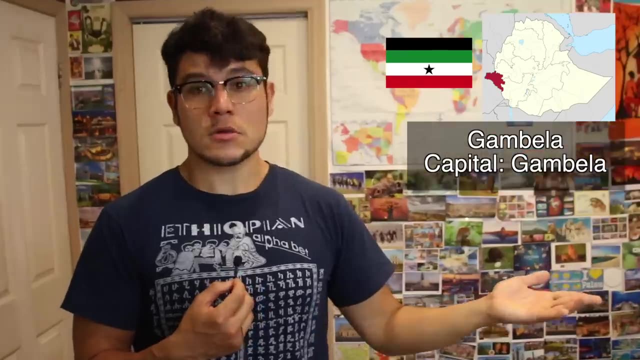 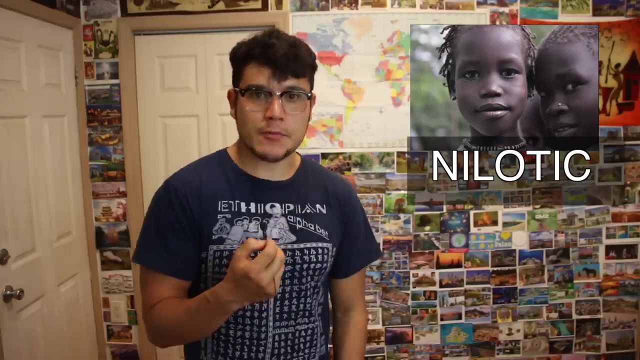 Many Arabs and Europeans opened shops and businesses in the 20th century but eventually moved out, but you can still see the remnants. Gambela capital, Gambela, The westernmost region of Ethiopia, juts into South Sudan and, just like South Sudan, the predominant people group here are Nilotic. 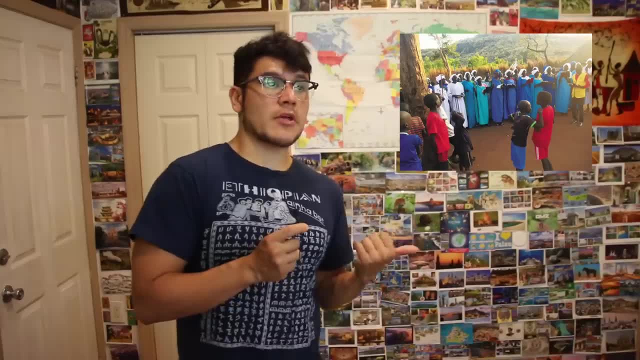 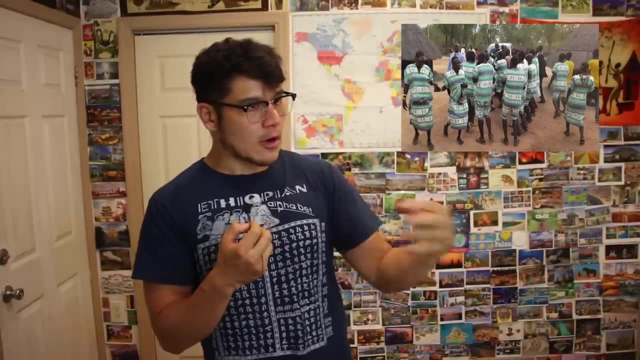 the largest groups being the Nuer and the Anuak. The majority of the population here is Christian, mostly Protestant, at about 70%. This place sits on the humid lowlands and whenever people come from like Addis Ababa or anywhere outside, 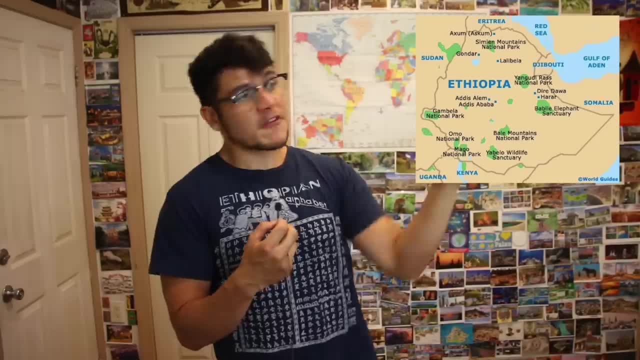 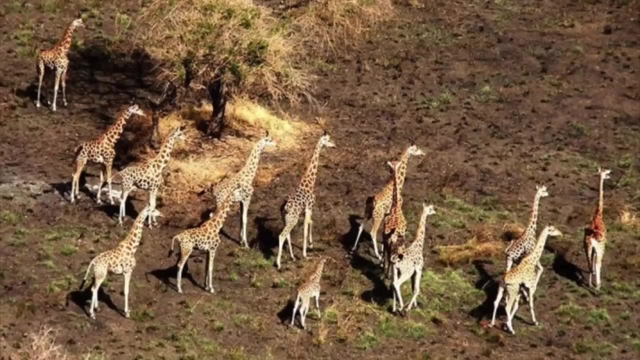 the people are always like: uh, it's a highlander. that's what they say. Almost a fifth of the land area of this region is made up of the Gambela National Park, which has one of the highest concentrations of flora and fauna in the country. 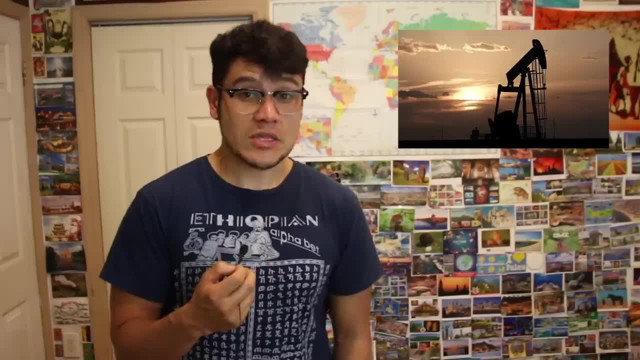 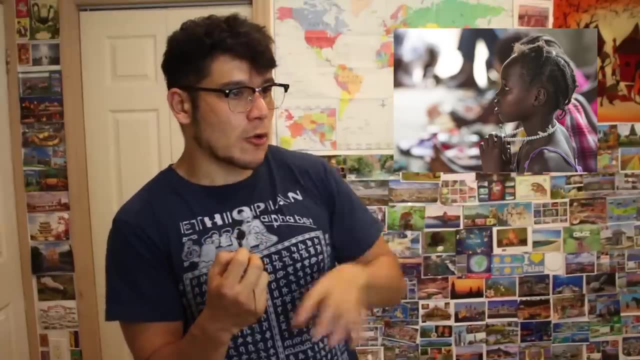 This is also the site believed to have oil in Ethiopia. In 2003, they signed a deal with the Petronas Company in Malaysia for drilling. But yeah, in any case, it's kind of like the Nilotic link between Ethiopia and South Sudan. 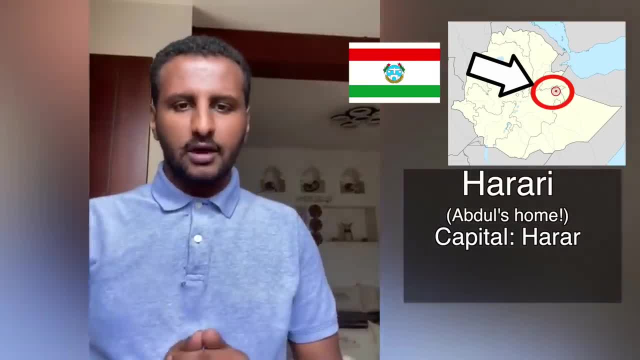 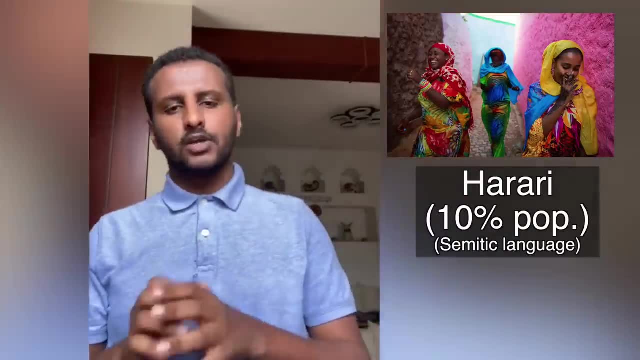 And for the next one, Abdul Harare, my home region capital, Harare. This is the smallest region and lowest in population. It almost acts like a charter city, but it isn't. It's still a region, home of the Harare people, a Semitic group. but we only constitute about 10% of the population there now. Historically this area had had some problems with former Ethiopian emperors and there has always been some kind of conflict, as we used to have our own ruling sultanate and emirate system. 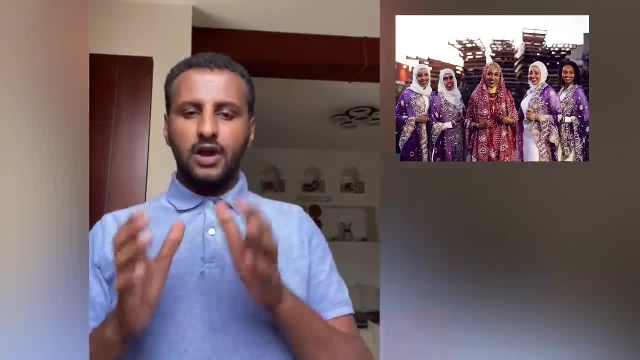 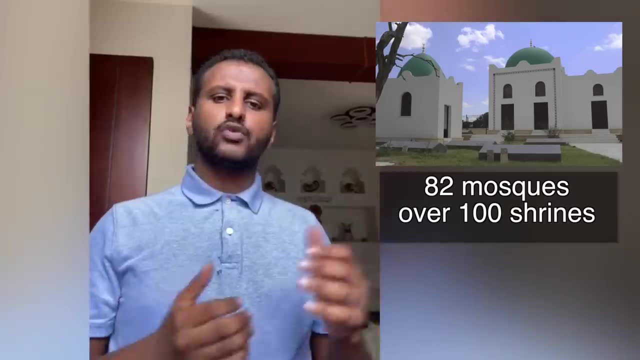 Christians and Muslims are about equal in population, but Islamic culture is very noticeable. Harare is considered the fourth holiest city in Islam. Yeah, in Ethiopia There are 82 mosques, 10 of which date back to the 10th century. 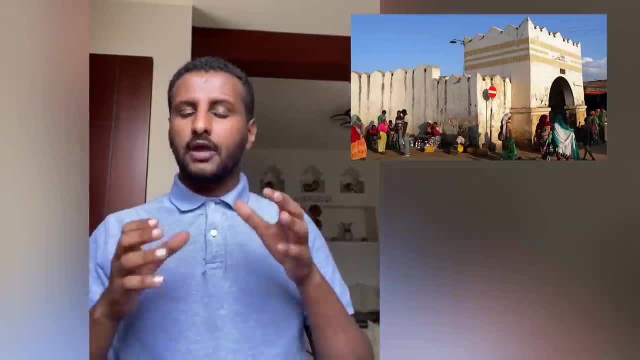 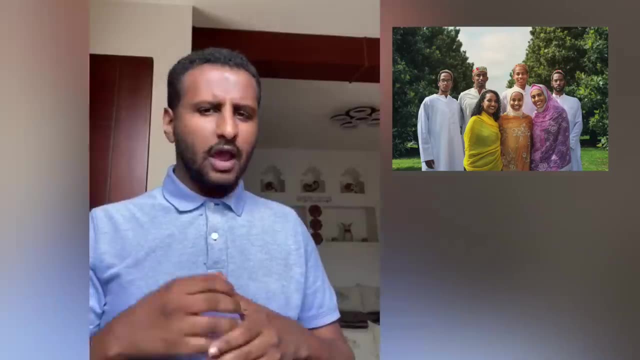 and over 100 shrines. As a trade city, there's a strong Arabic influence in the Harare people. You still see Arabic architecture and at one time the language was written in Arabic And our language is very similar to Swahili. 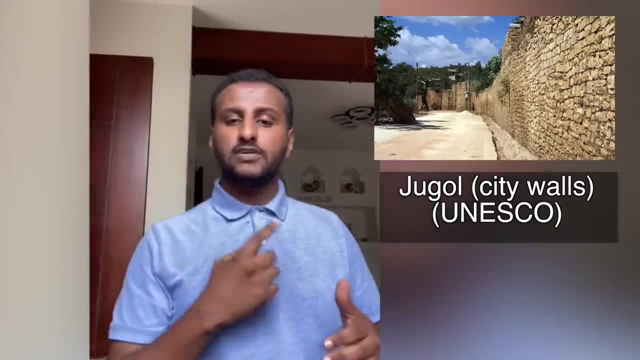 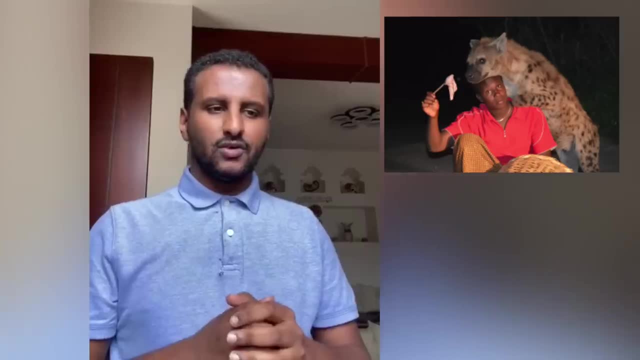 The main city of Harare is famous for being fortified by Jagol, a defensive wall that is registered as a UNESCO heritage site. And finally, Harare is also famous for a long-standing tradition of feeding hyenas. So the people in Harare have kind of developed a unique symbiotic trust relationship. 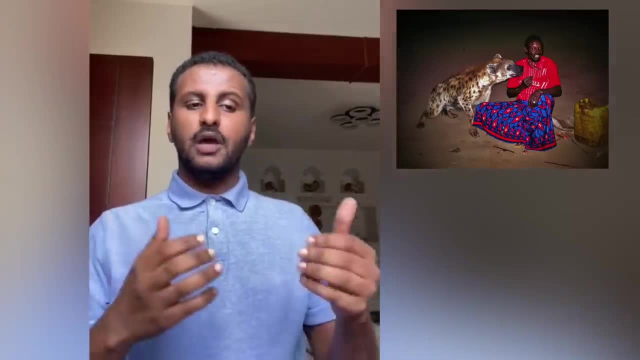 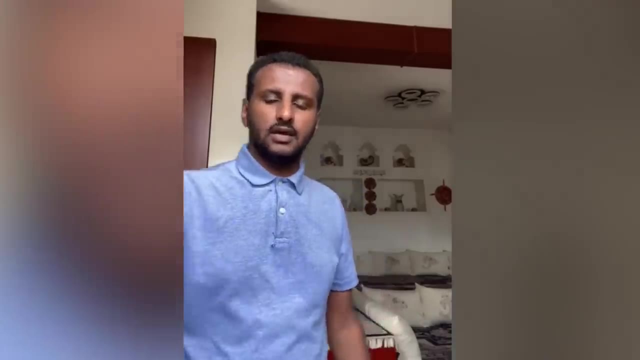 between themselves and the hyenas, And at night time the hyenas come and are fed raw meat, But this has turned into a show for tourists in recent times. By the way, this is what a traditional Harare room looks like. It's called Gegar. 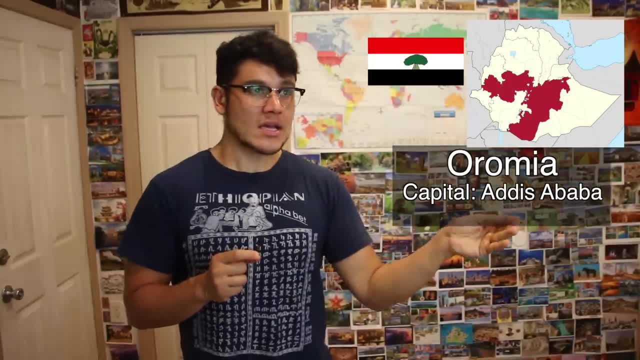 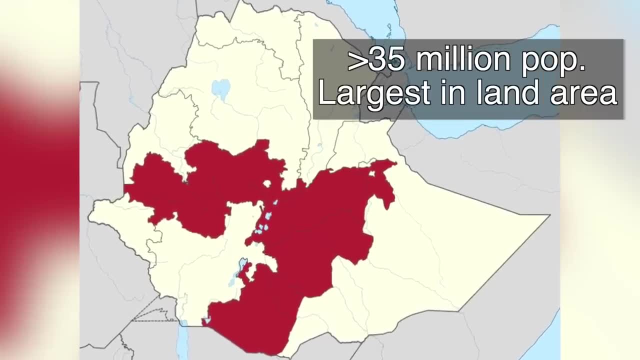 Oromia. Addis Ababa, the capital of the country, also acts as the capital of Oromia. Spread throughout much of the south west and center part of the country, it is the largest inland area and the largest in population. 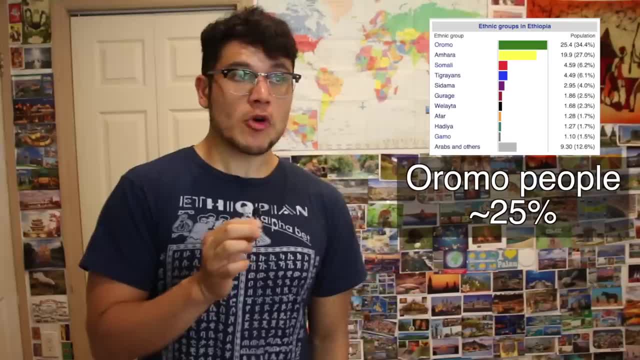 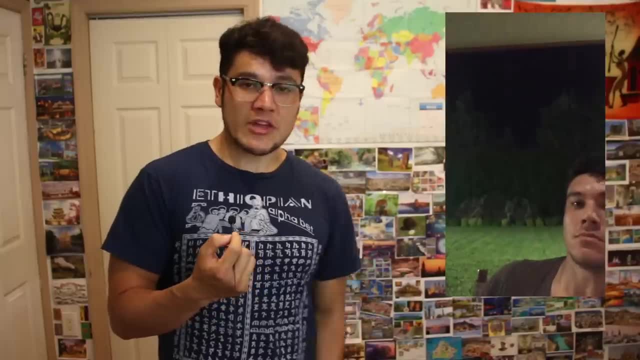 It is also the most populous subnational entity in all of Africa. The Oromo people within themselves are the largest ethnic group inside of Ethiopia, taking up about a quarter of the entire population. When Caleb and I were in Ethiopia, we had the pleasure to actually check out this area too. 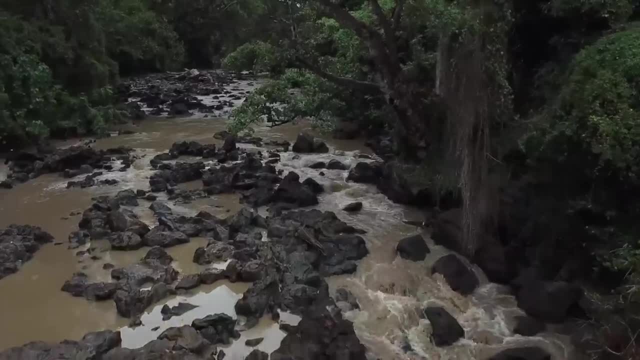 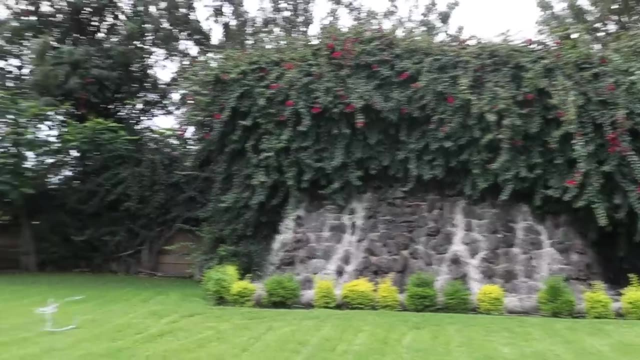 We went to Adama, which sits right on the East African Rift, So many of the rivers and lakes have geothermal activity. We were lucky enough to jump into a natural hot spring where wild monkeys crawled around stealing food. We visited a friend's house. 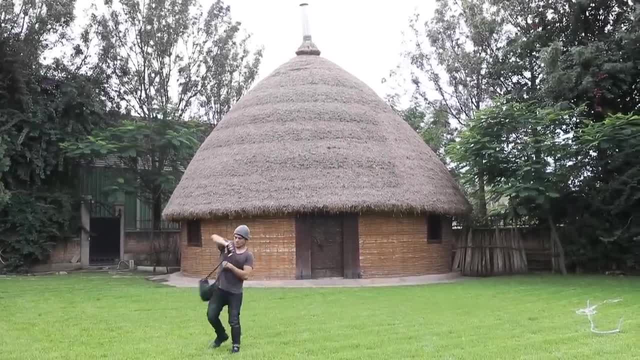 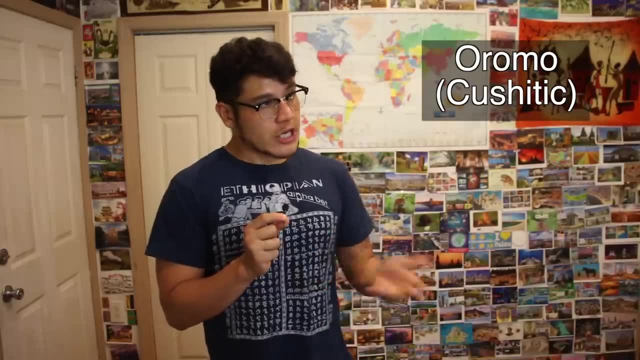 from the Goraga tribe. He had a traditional Gojo house in his backyard. Inside you could see the living units. It was really cool. I put all of this on my Instagram highlights. You could check it out if you want. The Oromo language is a Kushitic language related to Somali. 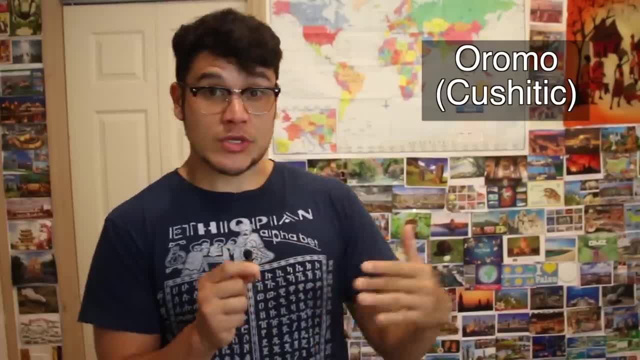 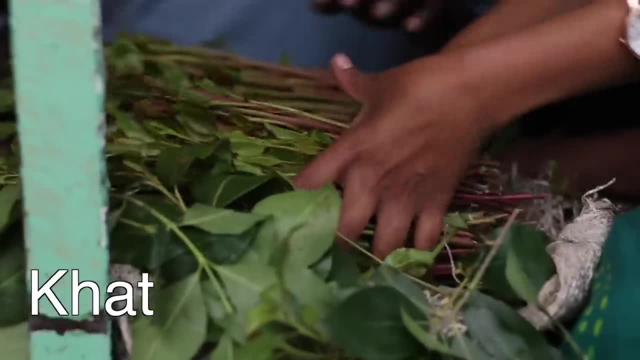 It is written in the Latin alphabet so you'll see that a lot on the street signs Oromia has a ton of resources, you know: gold, agriculture, minerals, cattle, chat. Oh, my Ethiopians love chat. You'll see like chat stalls everywhere in Ethiopia. 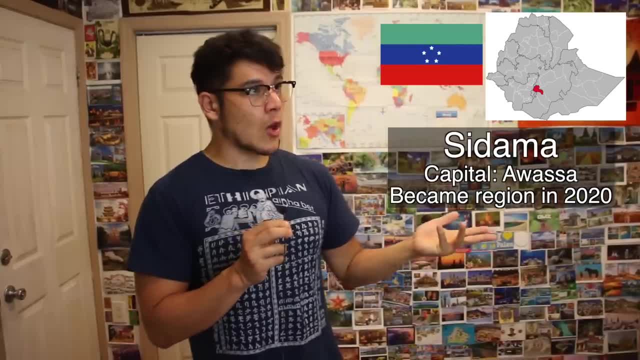 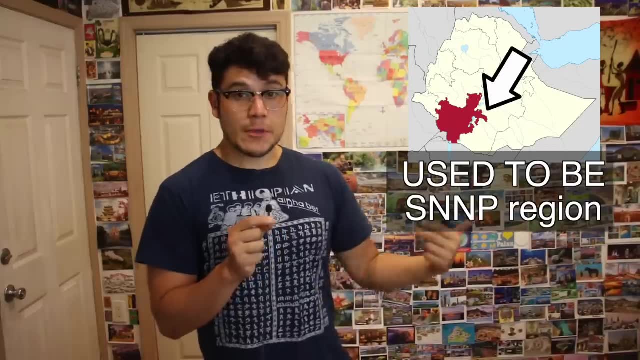 Holy crap, they are addicted to that stuff. Sidama capital, Awasa, Now remember. this is the newest region, that just joined in June of 2020.. They used to be part of the Southern Nations nationalities and peoples region but, like with a landslide, 98.5 in favor vote. 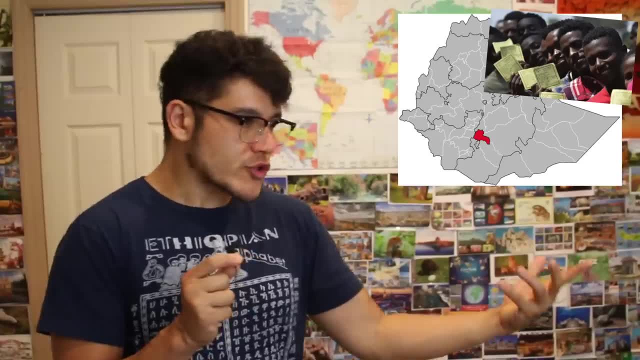 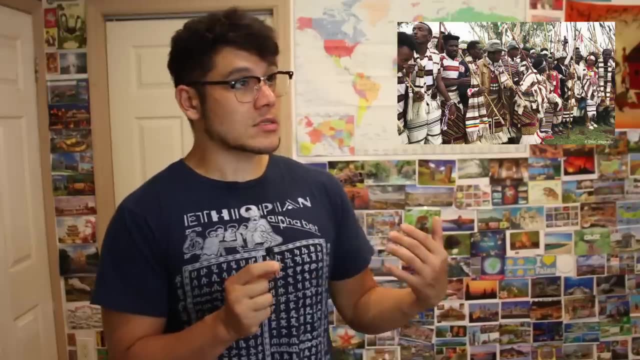 they seceded and became a region. They got upgraded from zone to region, Predominantly inhabited by the Sidama people, whomps forthwith are a Kushitic people group. Historically they have their own kingdoms, most notably the Kefa kingdom in the 1400s. 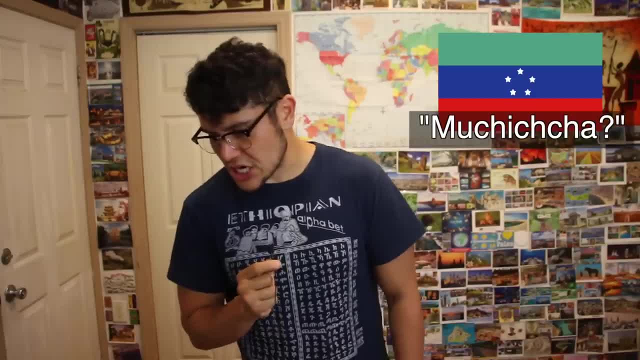 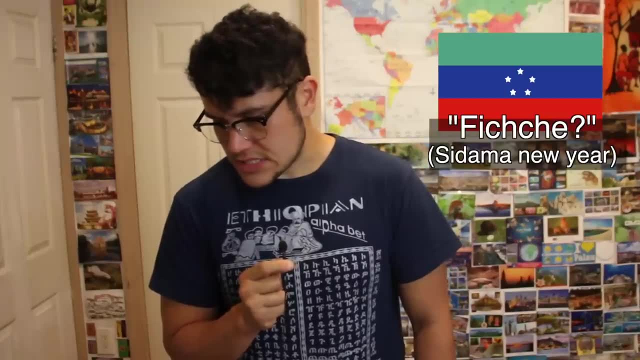 These kingdoms were ruled by a. what does it say? The Muchicha, which was like a king, but was nominated by family and would be presented and coordinated at the Fichche or Sidama New Year's ceremony. Hey, I'm learning alongside with you. 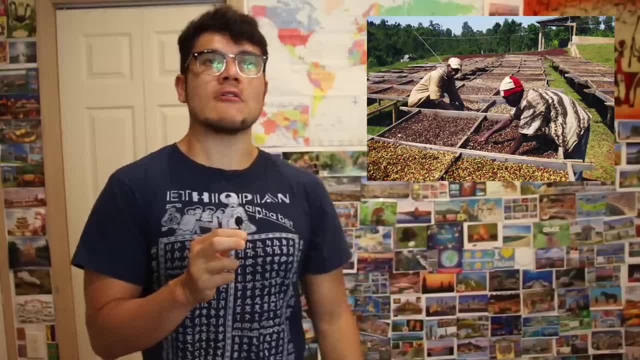 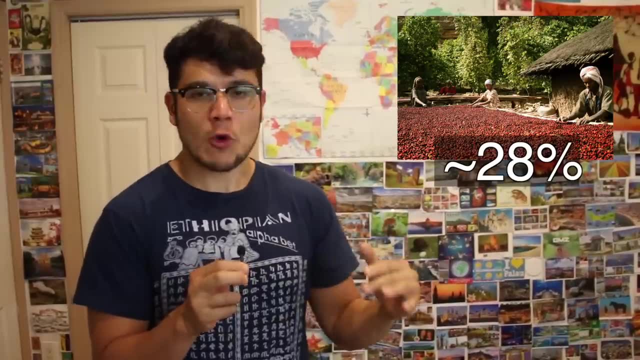 And essentially these people are kind of known for being the coffee people of Ethiopia. They alone, in their own region, make up about 28% of the entire Ethiopian coffee output. They produce a lot, which was one of the key determining factors on why they wanted to become a region. 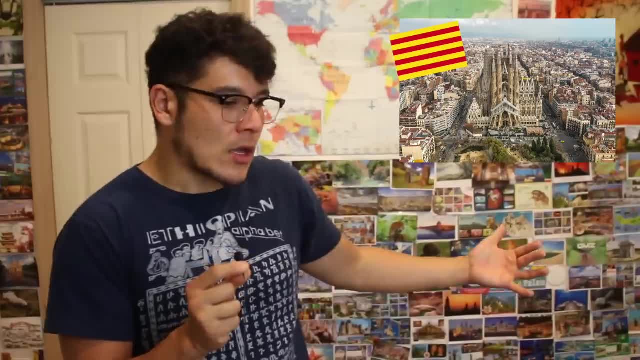 and they broke away. I mean, it's kind of like the Catalonia thing. It's like we make a lot of money, we're tired of holding down the other people. I guess, yeah, Sidama is kind of like the Catalonia of Ethiopia. 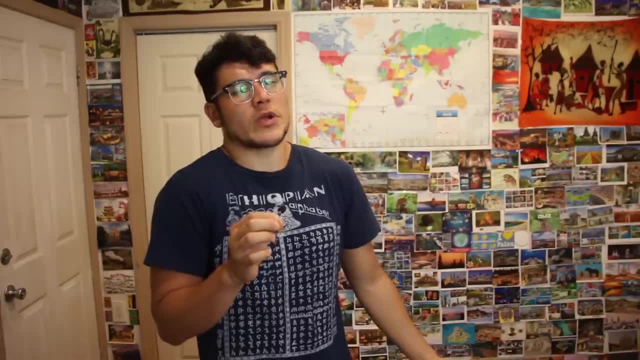 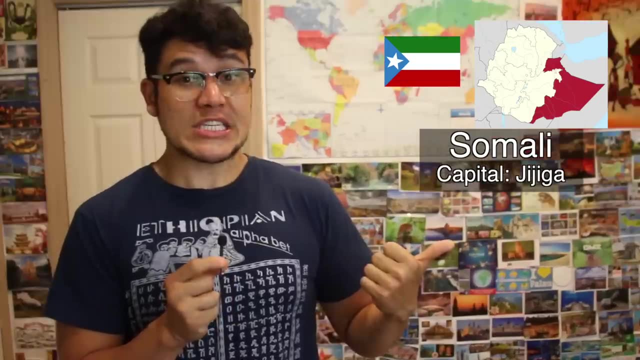 Don't quote me on that. I mean you probably will, but I mean I'm just making very weak comparisons. Whatever, moving on, Somali, Not to be confused with Somalia, the Somali region of Ethiopia, Capital, Jijiga. Love that word, Jijiga. Yes, the majority of people here- at about like what? 98%- are ethnically Somali And yes, that means they have pretty much the exact same ties and culture to the Somali people in Somalia. 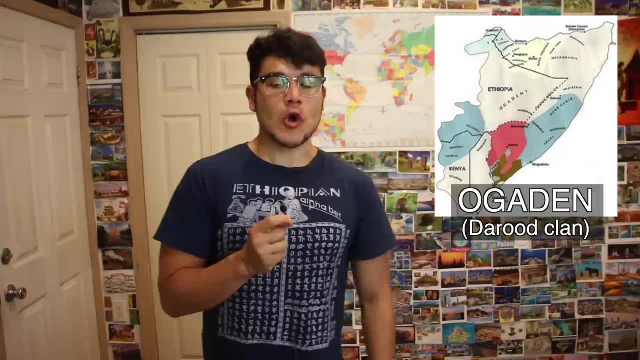 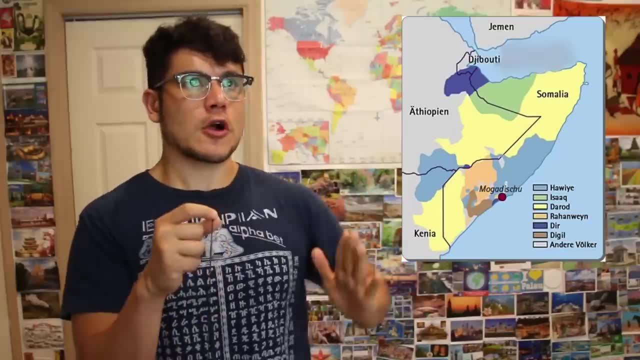 or the self-declared state of Somaliland, But that's another thing I'm not going to get into that. Located in the historic territory of Ogaden, part of the Darod clan, the Somali region of Ethiopia is considered part of the larger, Greater Somalia. 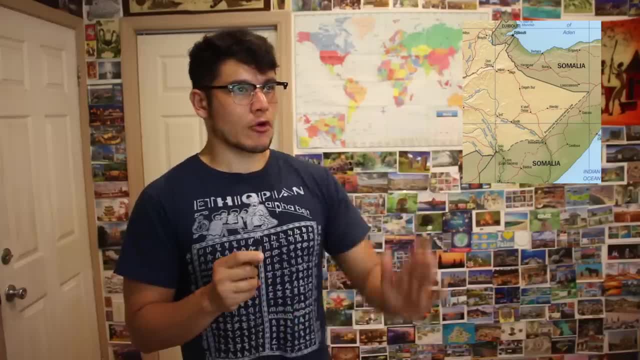 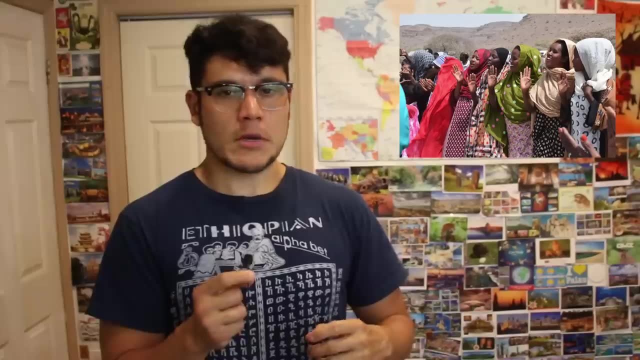 or the area of Africa where all the Somali people live. Even their border with Somalia isn't exactly completely agreed upon, and people living close to the border don't even bother to like demarcate which country they live in. Many people who live in Somalia will actually just cross over. 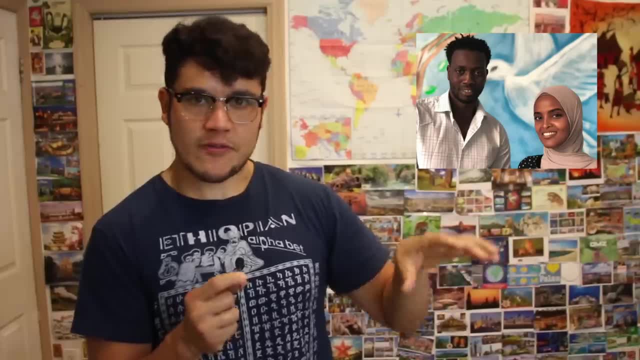 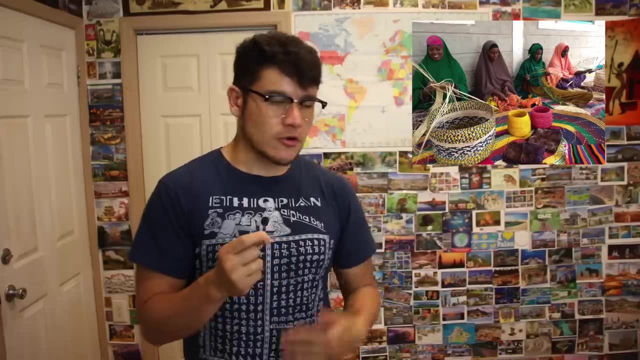 and like apply for Ethiopian citizenship by using their family to vouch for them, because the Ethiopian passport is more powerful than the Somali one. In any case, the vast majority of people here are Muslim. Somali culture, if you don't know about it. 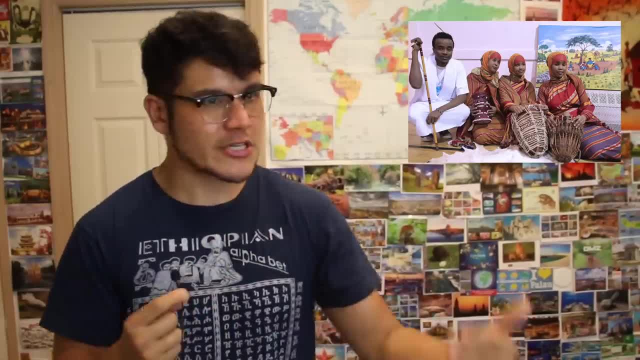 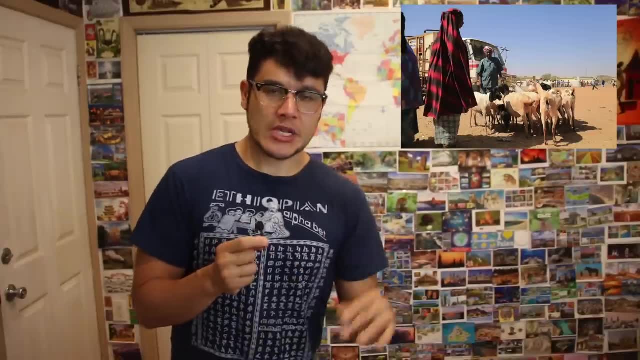 is just filled with way too many vibrant cultural traditions and food and it's just too much to talk about. We'll talk about it in the Somali episode, But in a nutshell it is heavily rooted in pastoralist culture. as much of the land as arid, dry shrubland. 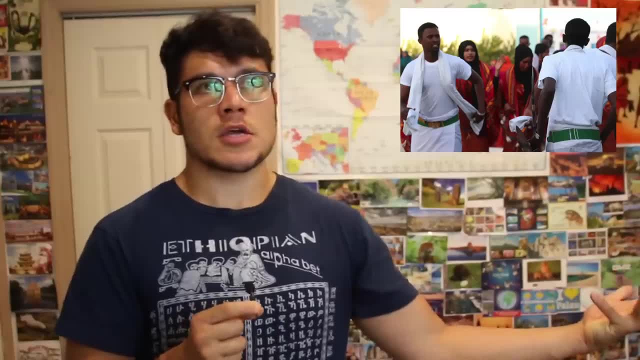 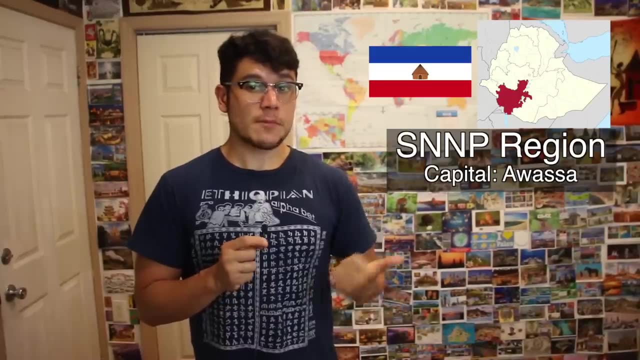 But yeah, it's basically Ethiopian Somalia, for lack of a better term, Don't quote me on it, you will quote me. I'm ruining my life Moving on The- That's literally what it's called. They share their capital, Awassa, with the Sidama region. 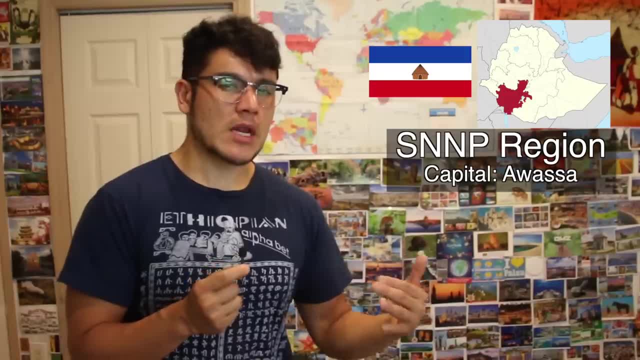 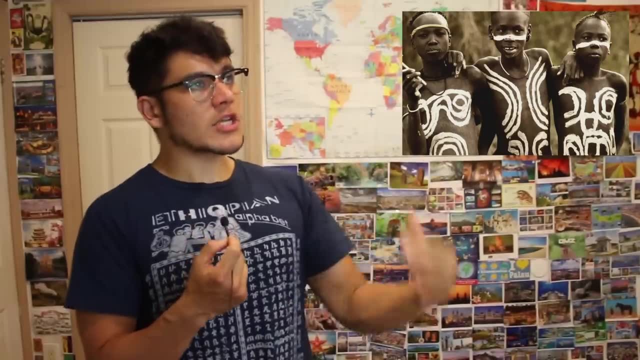 that, just you know, got a new region status. They're talking about potentially maybe getting a new capital, but for right now, Awassa acts as the capital for both of them. In any case, this is the most ethnically diverse area in all of Ethiopia. 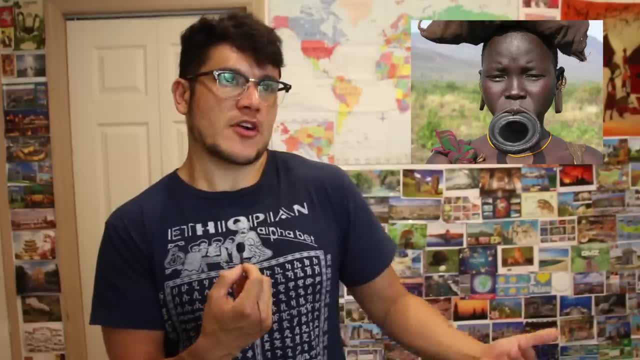 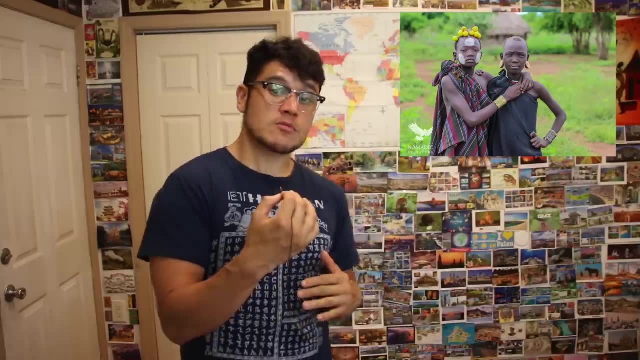 Most regions in Ethiopia only have like a couple ethnic groups, maybe 10 max. This one has over 50,, some say over 80, depending on how you want to divide the subgroups. It is also Ethiopia's most rurally dispersed region. 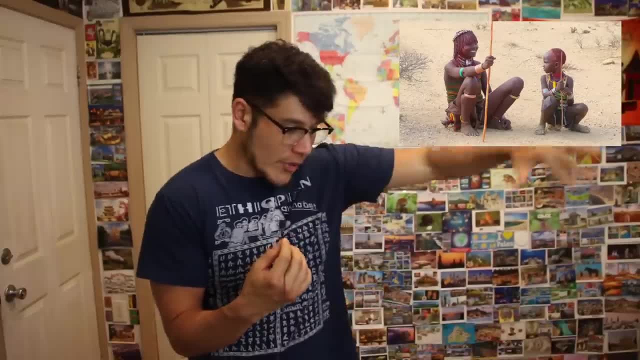 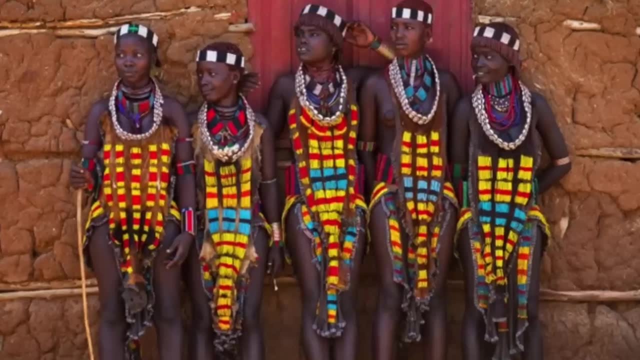 As about 90% of the population do not live in cities. They live on their own little plots of land in the middle of the countryside. 90%. can you believe that Here you find the most contrasting communities with different clothing, jewelry, lifestyles, celebrations and values? 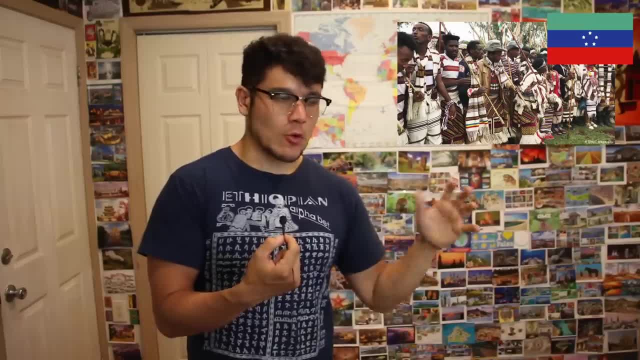 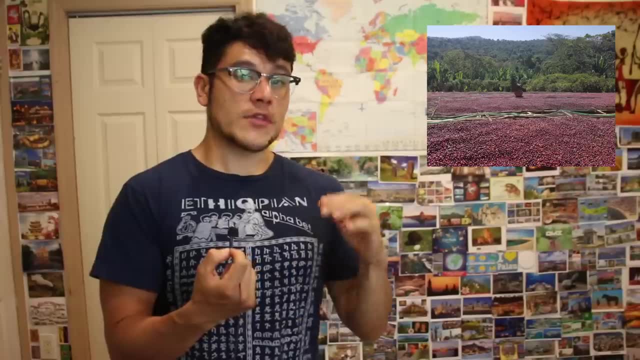 all within short distance from the next one. Prior to the breakup, the Sidama people were actually the largest group, at about 20%. Now that they aren't, the new largest group is the Welaita, at about 11% Now. this is actually the largest coffee producing area in all of Ethiopia. 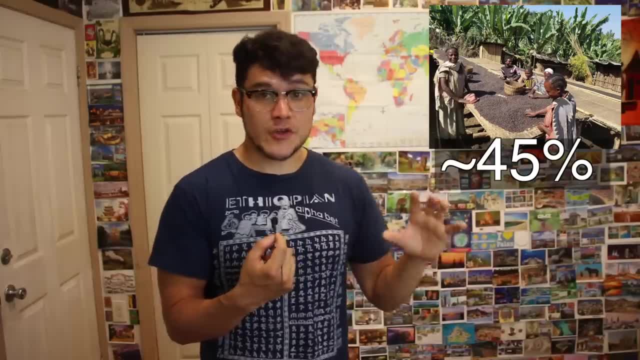 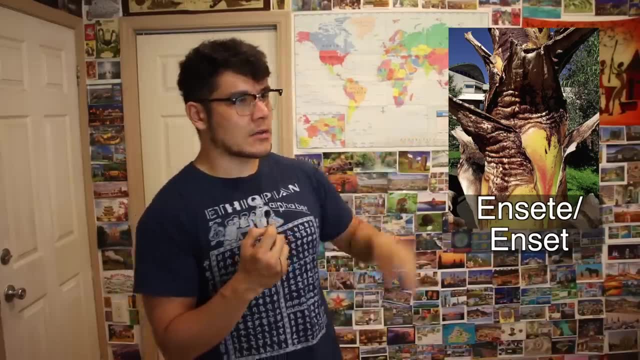 Sidama got 28%. This place has 45% of all of Ethiopia's coffee output production. They also grow some of the largest amounts of ensete, or Abyssinian false banana, which is actually cultivated for its trunk and stems. 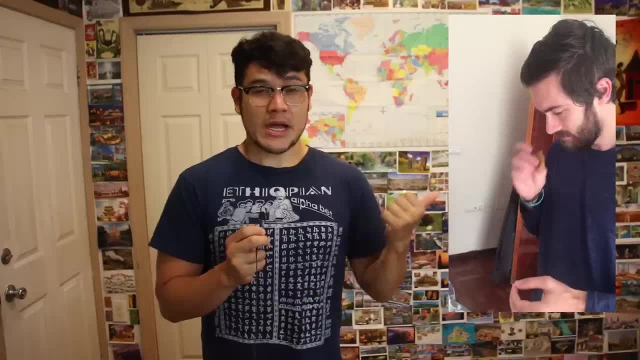 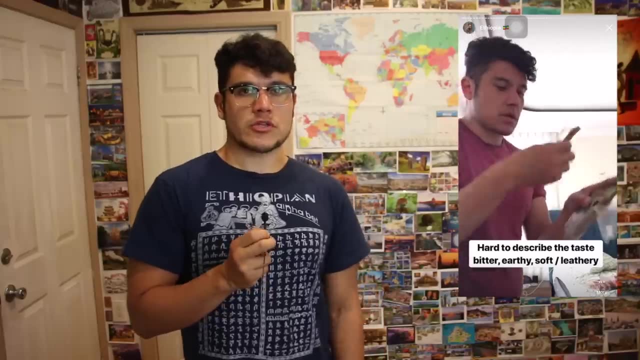 They mash it into a paste and make it into like a little circular disc. Caleb and I actually tried it. Caleb absolutely hated it. Even Abdul and the other Ethiopians we were hanging out with they didn't even like it. But me trying to be like the douchey, like I'm so cultured. 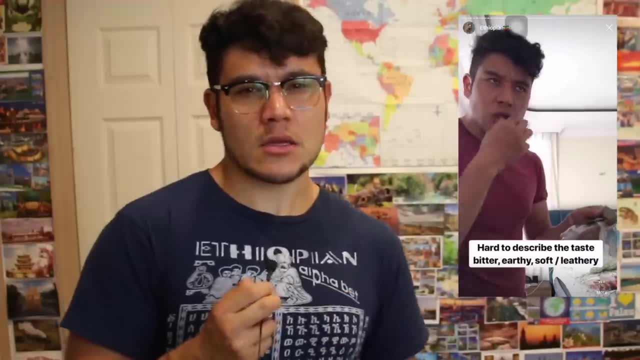 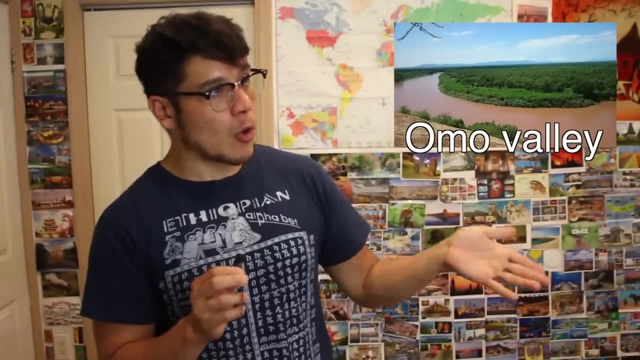 Like I'm all like, oh, it's good, it's good, But in reality I didn't really like it, I have to be honest. Anyhow, This place is also known for the world famous Omo Valley, with the Omo National Park and Omo River. 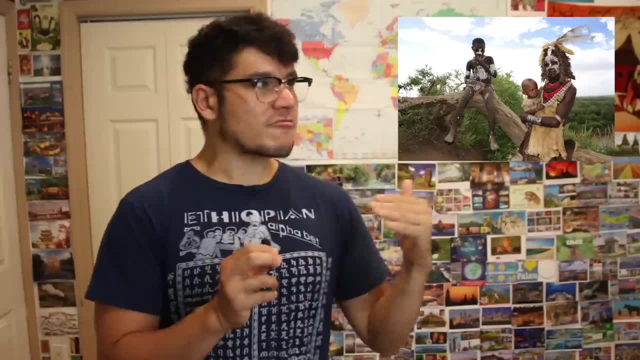 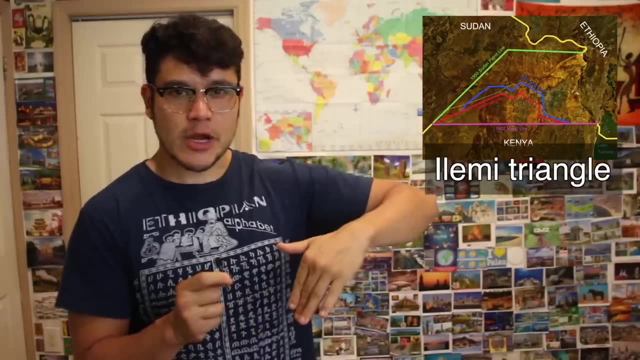 There are so many cultural villages you can visit where you can meet the native people. They also have a small piece of Lake Turkana on the border with Kenya And they are also on the border disputed area of the Ilemi Triangle with South Sudan. 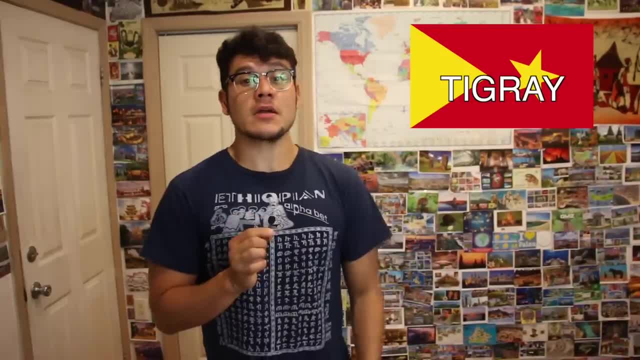 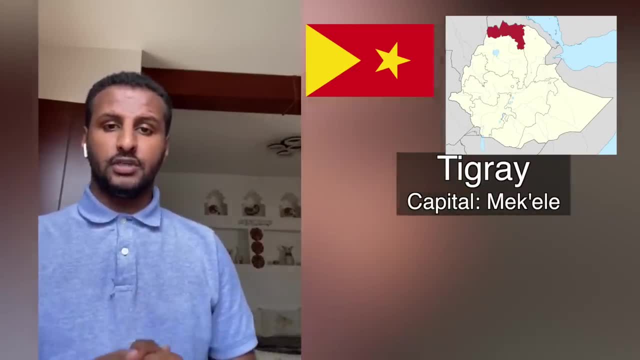 Check it out if you want a diverse experience. And finally, the Tigray region. And here we go again, Abdul, take it away. Tigray, Magali. This is the northernmost region. This is a very cool one. 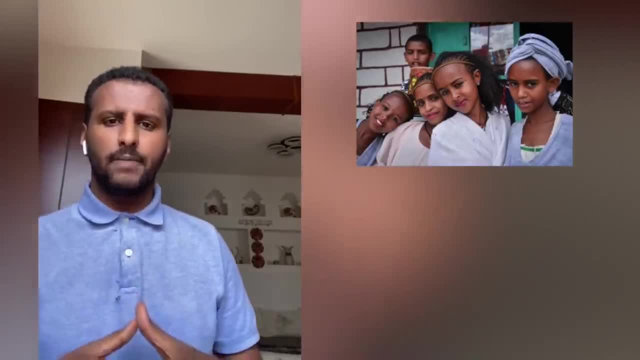 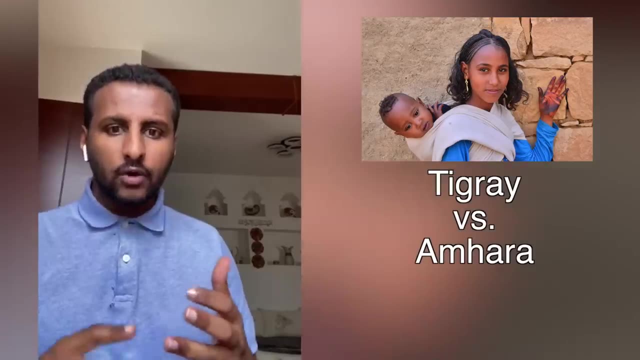 The area is inhabited mostly by the Tigray people, And they're basically the closest cousins to the Amharas, Both mostly orthodox, ethnically Habesha. Their languages are partially intelligible And they even write in the same script, the Ge'ez. 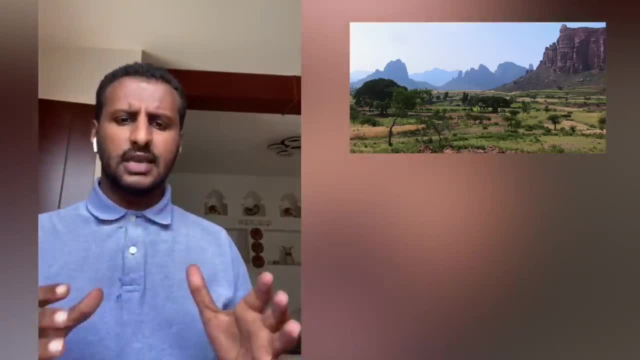 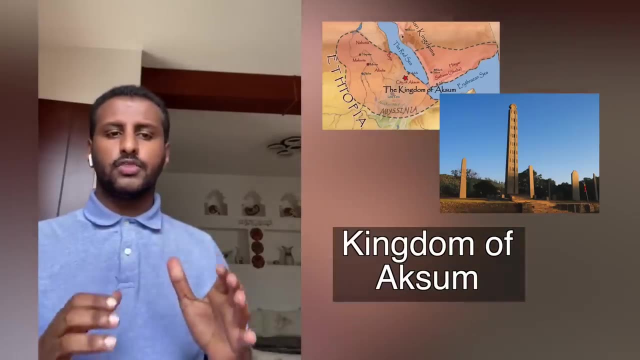 The Tigray region is blessed with some of the most contrasting landscape and historical landmarks. You have the upper plateau and mountains like Saramba and Ambalaje, But the most notable thing about the Tigray region is its landmarks and monuments that date back to the kingdom of Aqsa. 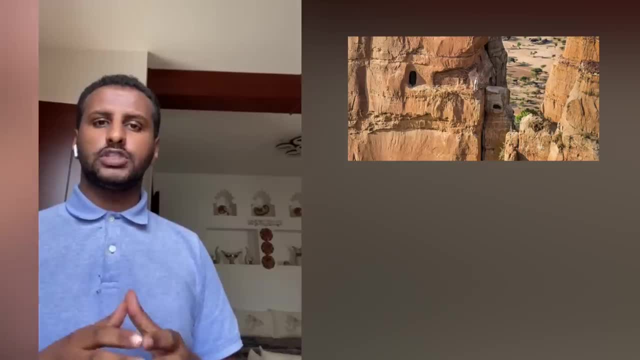 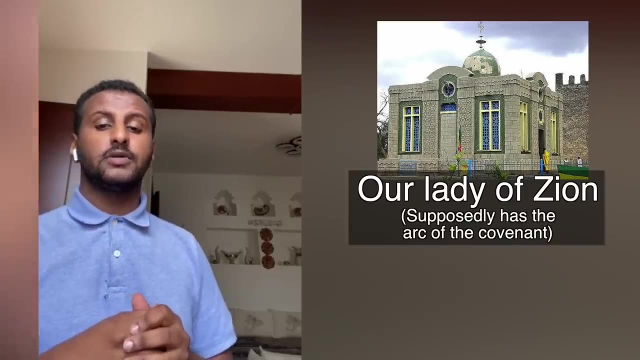 They were built around 1 century AD, Distinguished by its rocky architecture, in which entire buildings and churches were just carved out of the rock. This was where some of the earliest Ethiopian history begins, And archaeological sites pop up more and more over time. 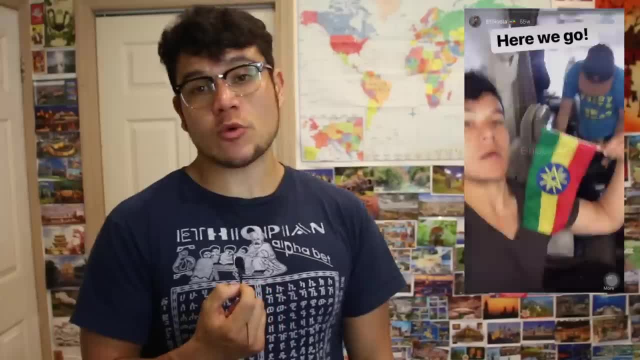 So yeah, there you go. Those are the regions and charter cities of Ethiopia. For what it's worth. I'm so glad me and Caleb got to have the experience to go there last year. The people were so super nice. They showed us around. 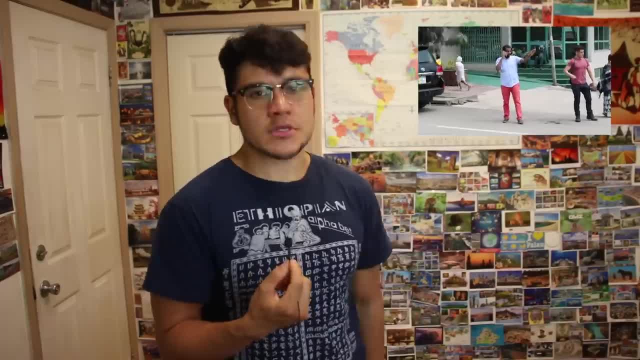 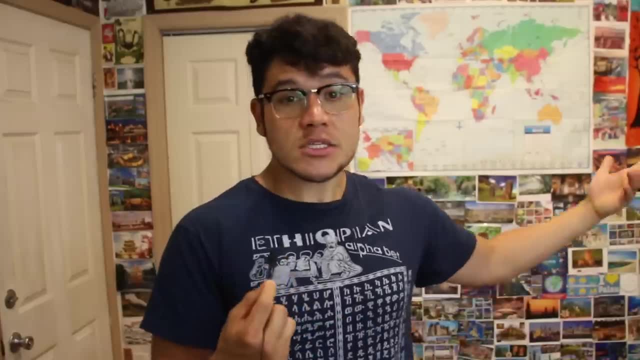 They were really proud of their country And I feel like I got a great experience. So what did I miss out on? If you are Ethiopian, feel free to write in the comments anything else I forgot to mention about the regions. Teach us. 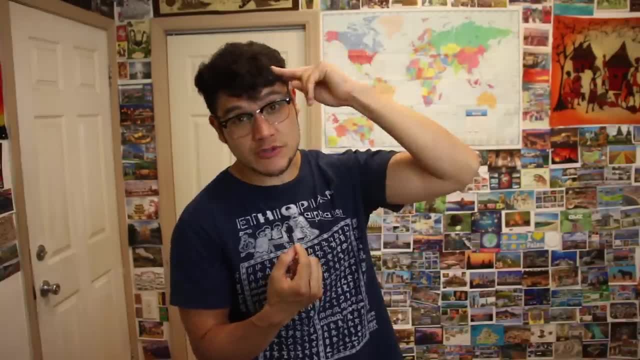 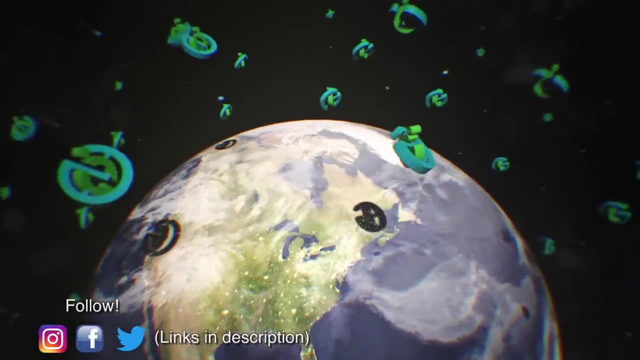 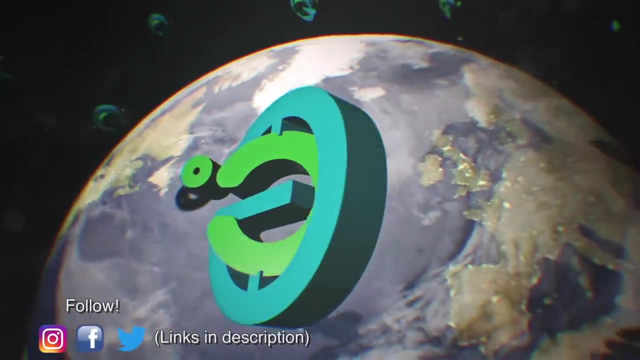 And yeah, thank you so much. Hope you guys have a good one. Stay cool, stay tuned. Bye, Bye, Bye, Bye, Bye. 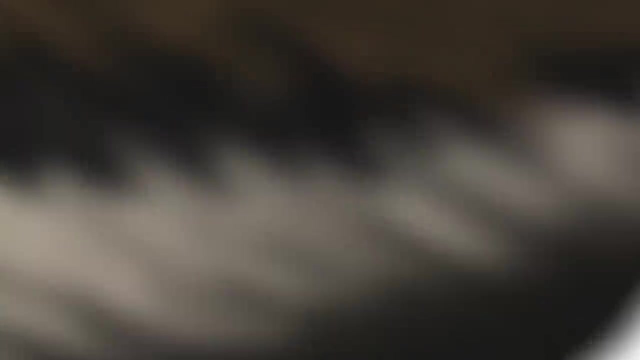 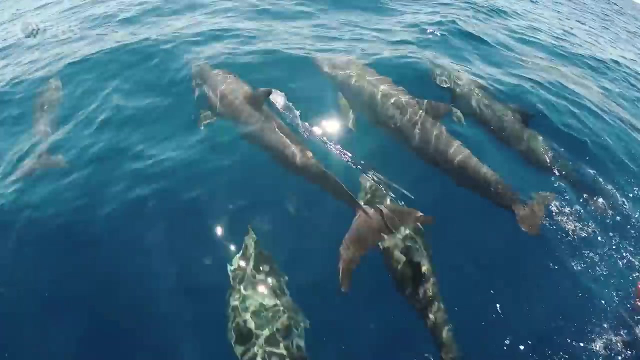 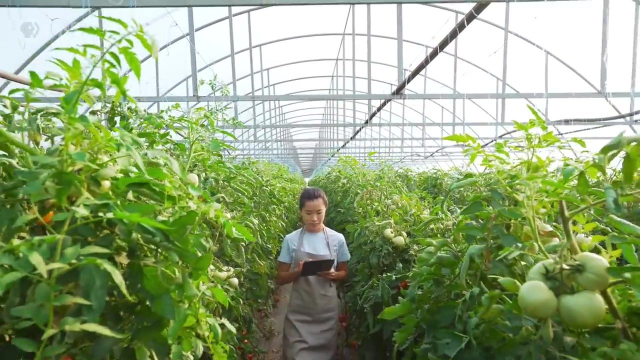 Thank you to Brilliant for supporting PBS. We mammals are very proud of being the big brains of the vertebrate world, with the largest brains relative to body size of any group. Our big, complex brains mean that mammals are frequently counted among the best problem solvers, planners, team workers and inventors that nature has to offer. 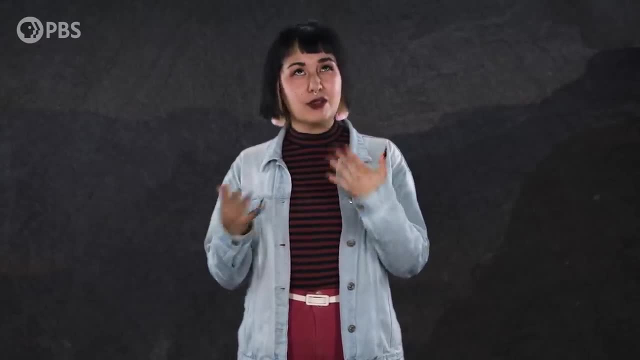 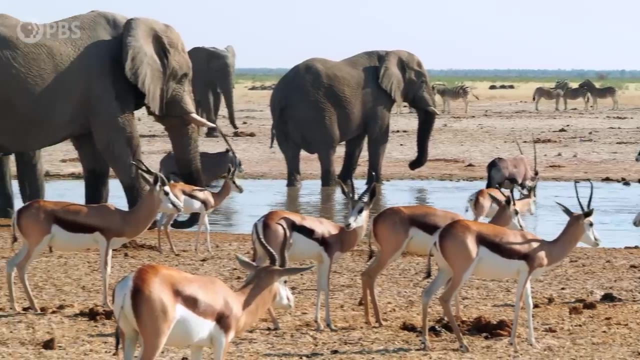 Of course, it tends to be us doing the counting, so there might be some bias there, And it's tempting to think of this feature as the key to our success. Surely we live in what's sometimes called the age of mammals, for a well-earned reason.